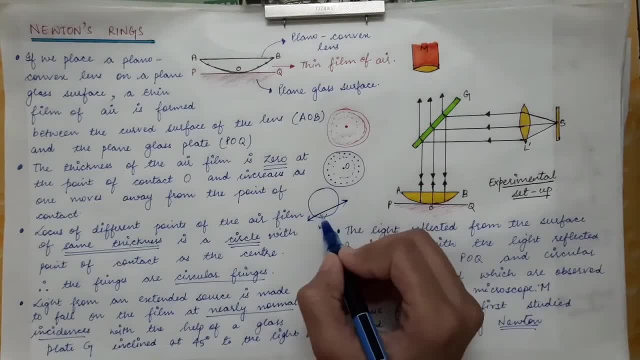 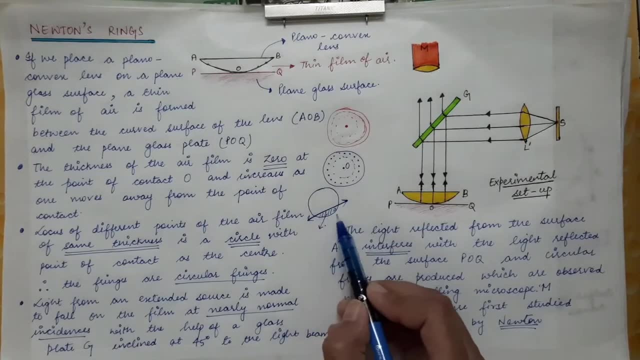 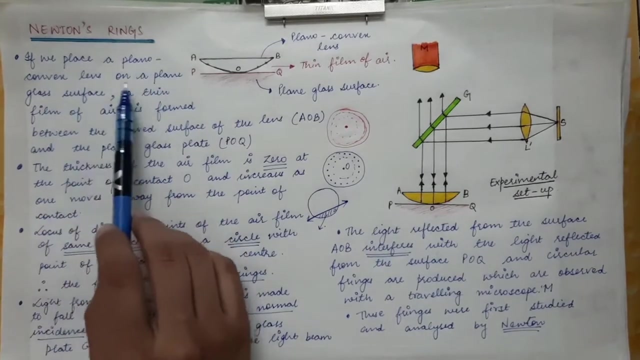 the plano convex lens. So this small section which is obtained. this is the plano convex lens And it is plain from the top and is curved from the downside. So if we place a plano convex lens on a plain glass surface, a thin film of air is formed. 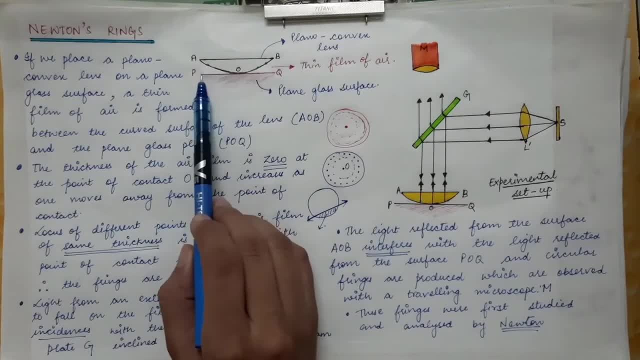 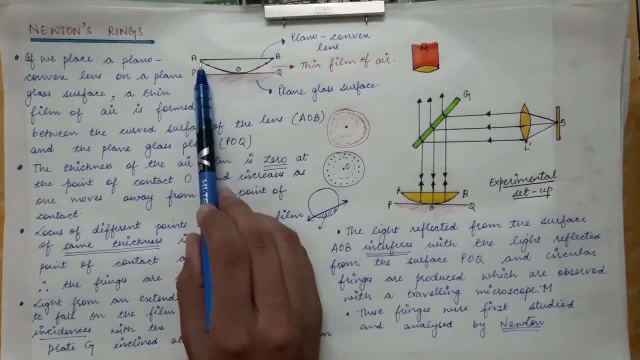 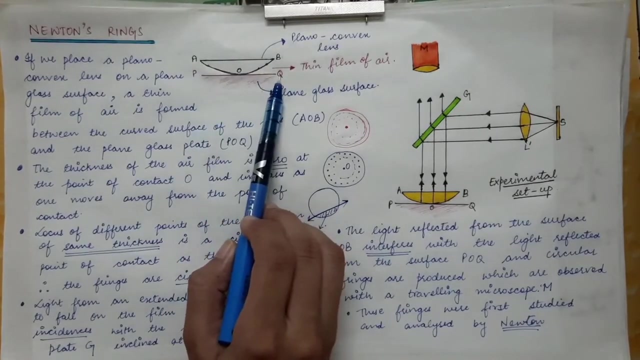 So the space between this curved surface and the plain glass surface, this empty space, it is filled with air. So a thin film of air is formed between the curved surface of the lens and the plain glass surface, and the thickness of the film it varies. 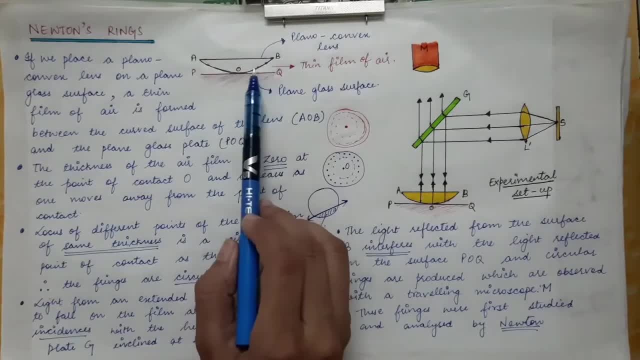 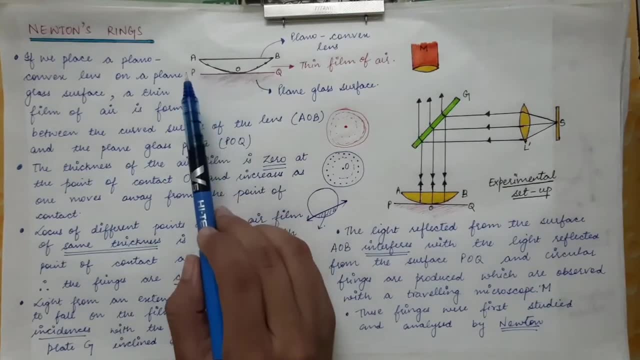 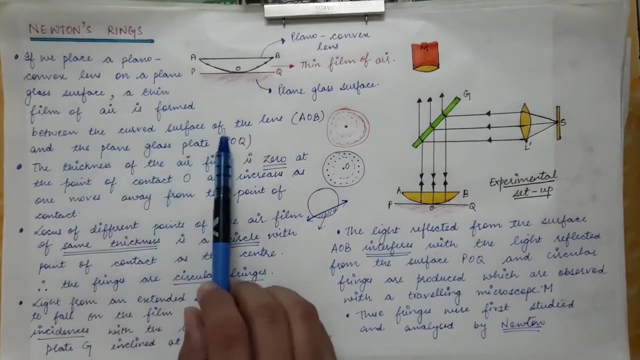 So you can clearly see that the thickness of the film it varies. The thickness is zero at the point of contact and as you move away from the point of contact the thickness of the air film it increases. So a thin film of air it is formed between the curved surface of the lens and the plain. 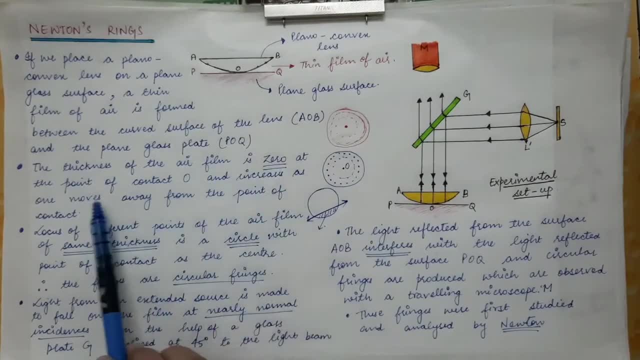 glass plate. The thickness of the air film is zero at the point of contact and it increases as one moves away from the point of contact. Now is the question that: why circular fringes? they are obtained due to this setup, So circular fringes are obtained. 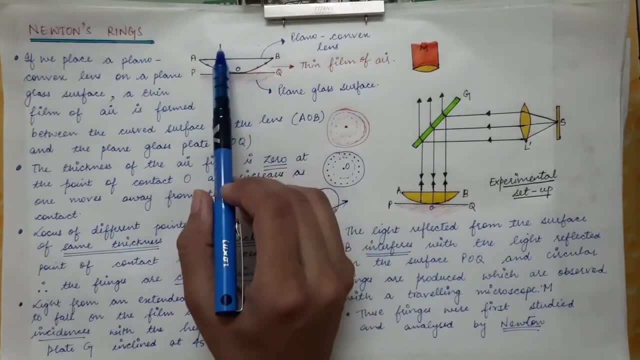 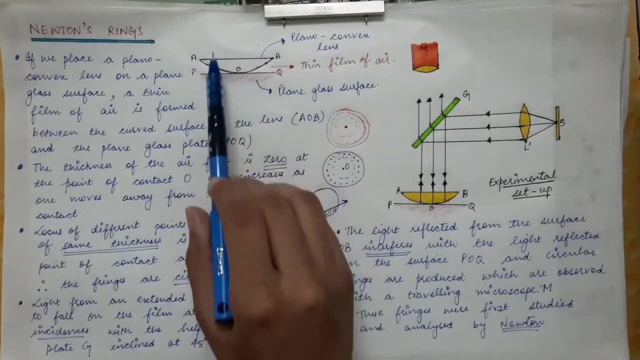 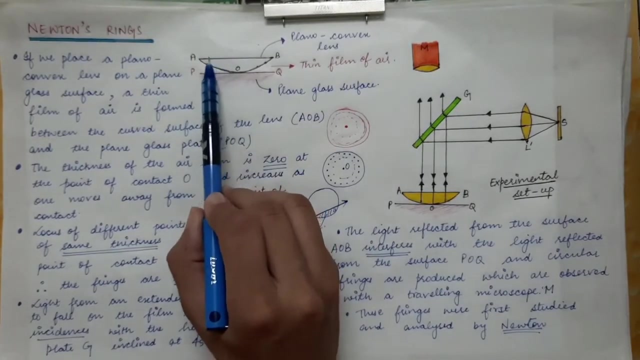 Now, what is the experimental setup of film Newton's rings? is that incident normal rays, or you can say the normal rays? they are made to incident on this particular setup, that is, on this lens, and the rays which get reflected. they are made to interfere with each other. 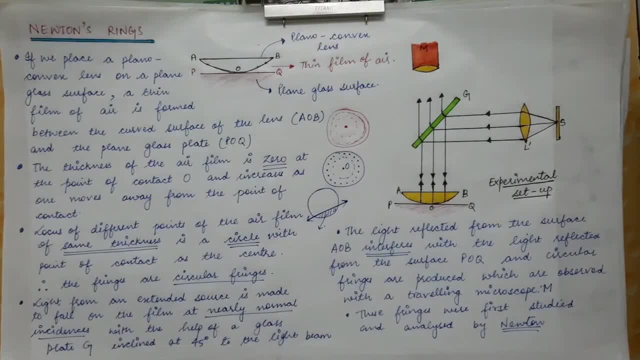 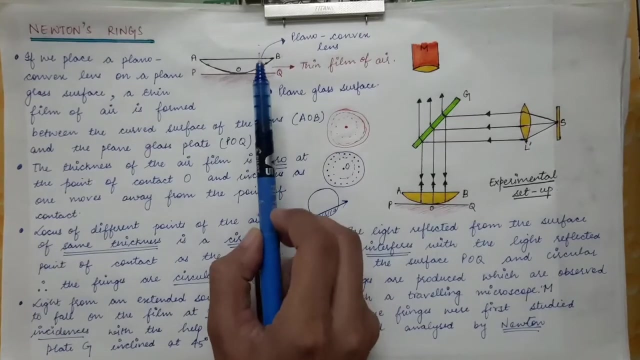 So the optical power difference between the reflected rays, it is given by 2 mu t cos r. So that is the general expression, 2 mu t cos r. it is the optical power difference between the two reflected rays. So let us say the light rays. they are incident normally on this lens and they get reflected. 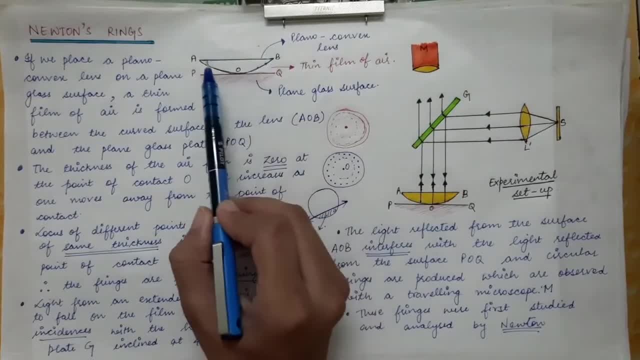 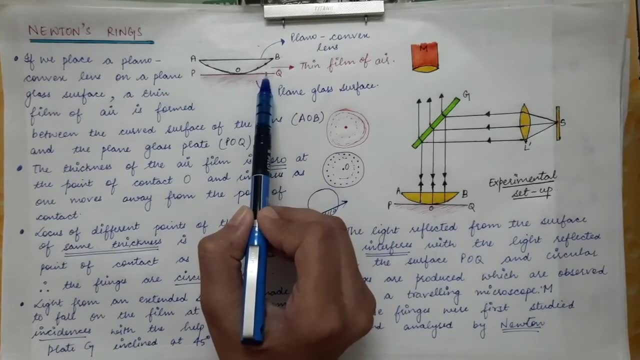 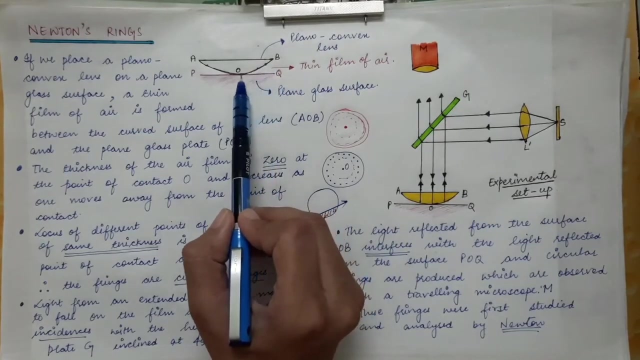 So they will get reflected. any incident ray, it will get reflected by this curved surface of the lens as well as it will get reflected by this surface of glass. So there are two surfaces of the thin film. this is the upward surface, top surface of. 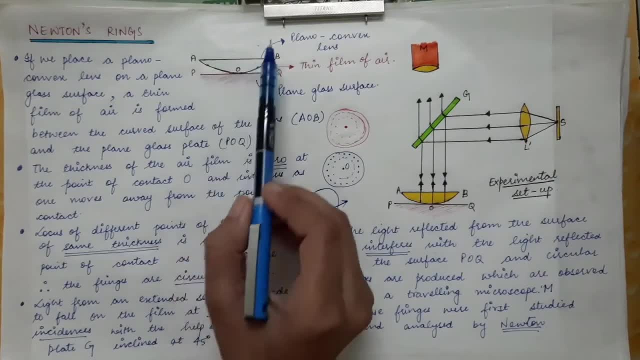 the thin film and this is the lower surface of the thin film. So when the light is made to incident on this lens, so the light it will get reflected from the upper surface of the thin film and the light it will travel through the air film. 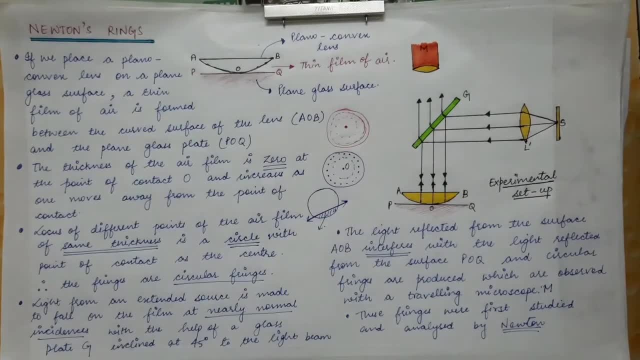 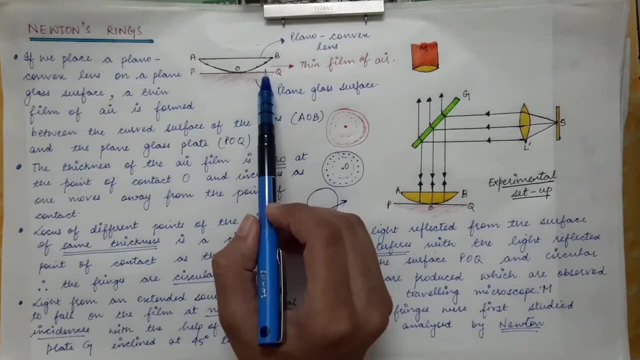 and then it will get reflected by the lower surface of the thin film. So those two light rays, they will interfere with each other. So those light rays, let us say they have a optical power difference of 2 mu t cos r. Now cos r will be equal to 2 mu t cos r. 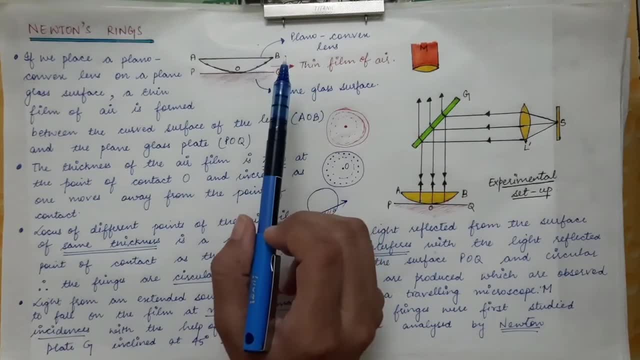 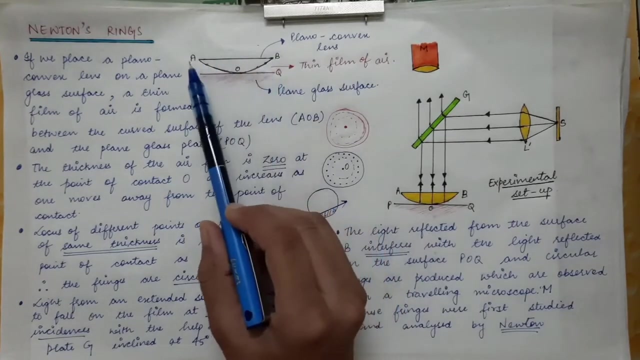 Now cos r will be equal to 1 because we are talking about normal incidence. So for normal incidence, i is equal to 0. therefore r will also be equal to 0. So the optical power difference will be just equal to 2. mu, t. and what are the type of fringes? 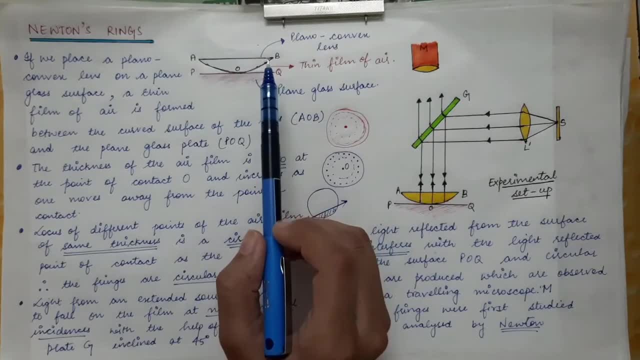 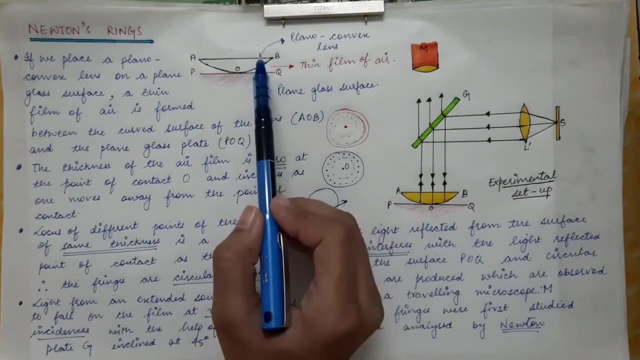 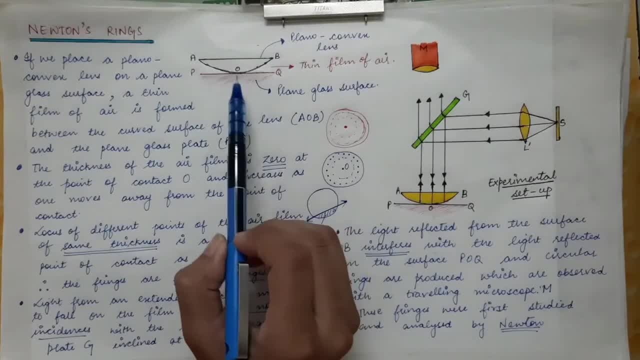 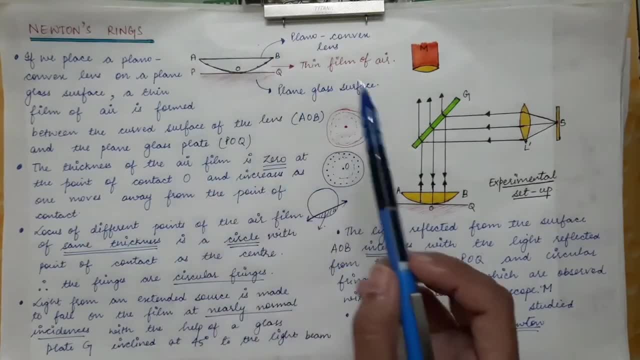 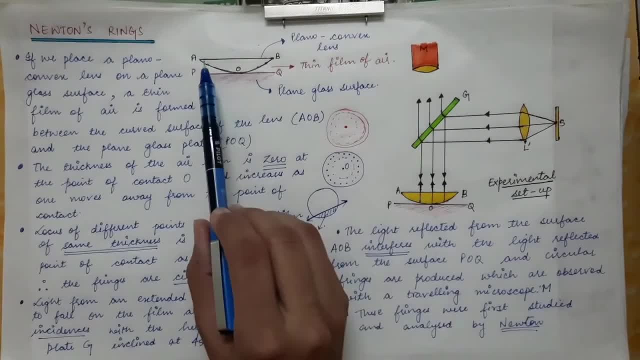 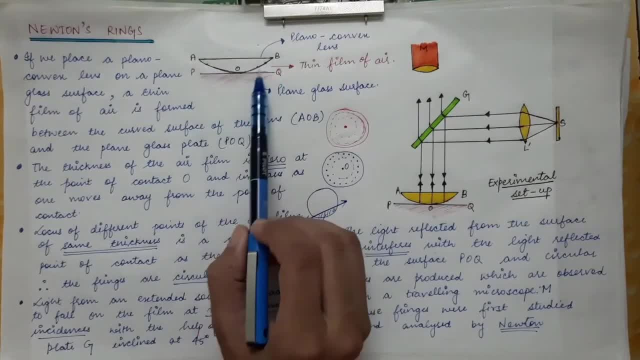 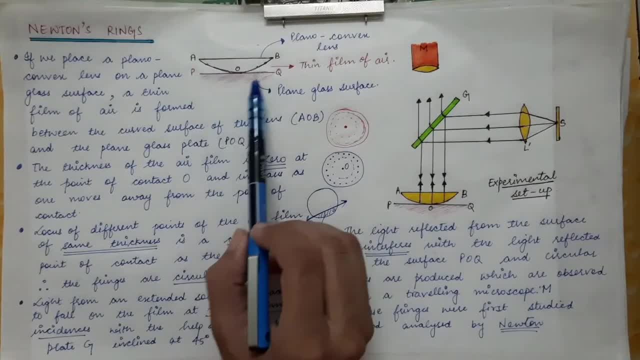 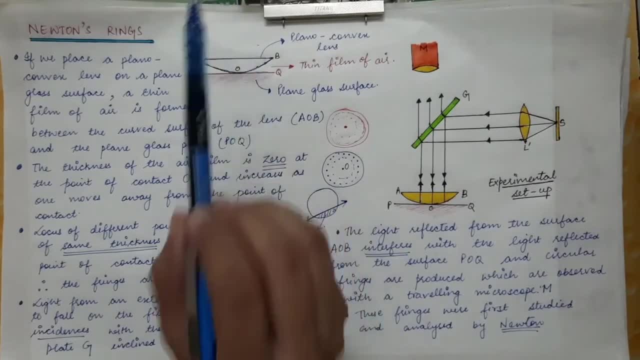 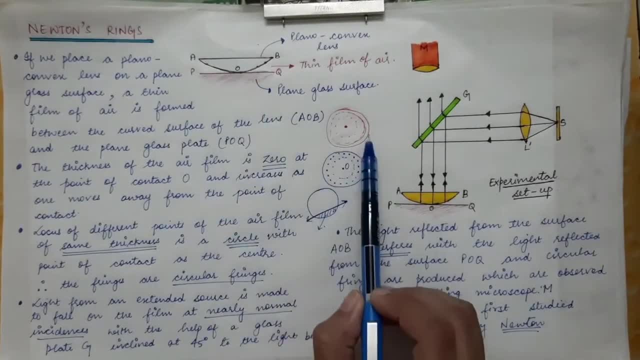 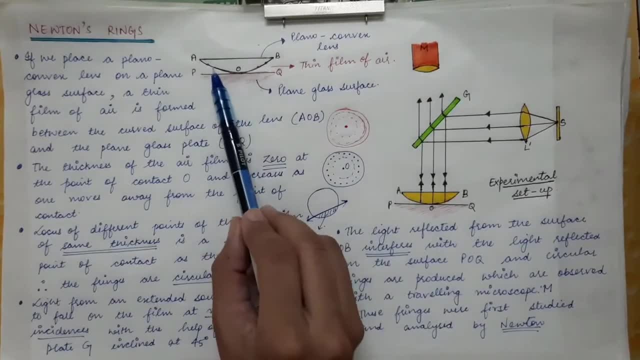 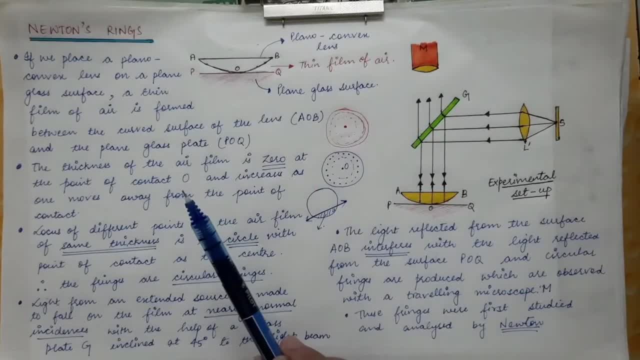 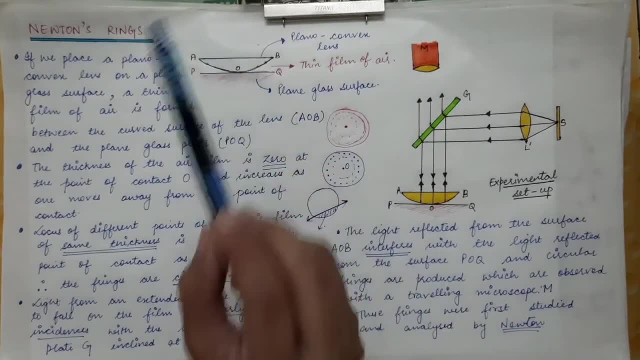 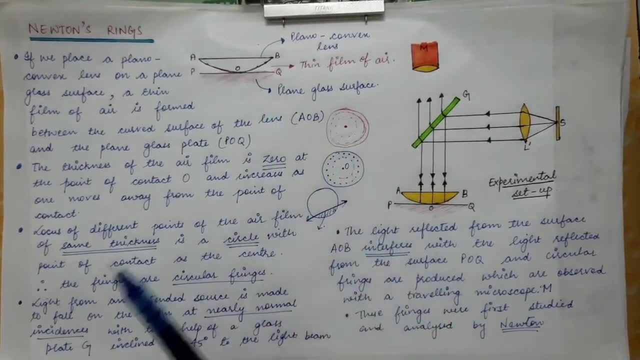 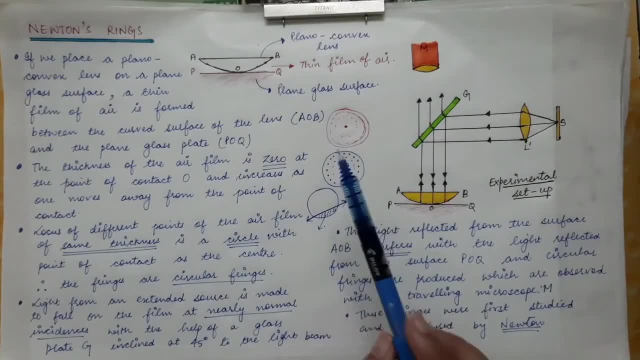 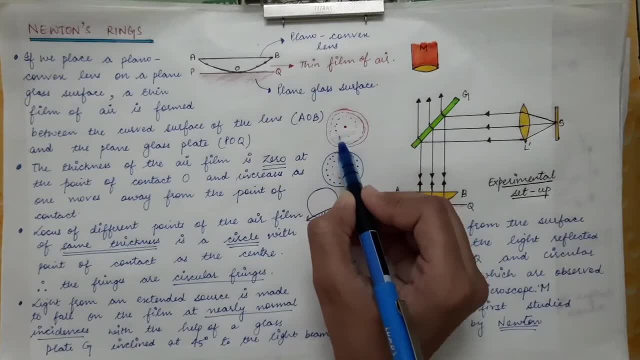 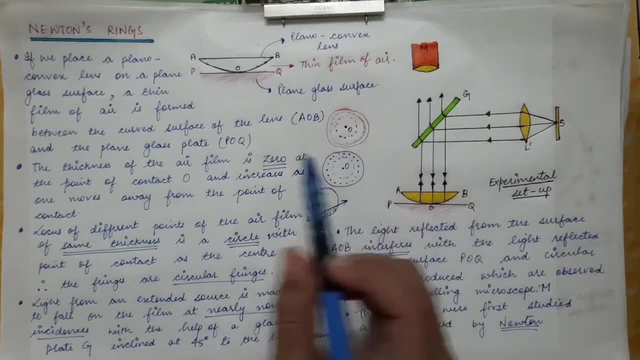 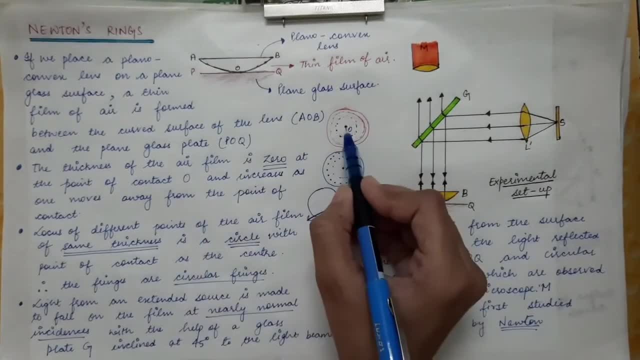 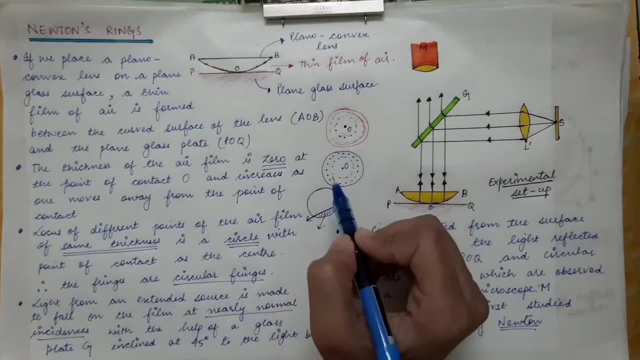 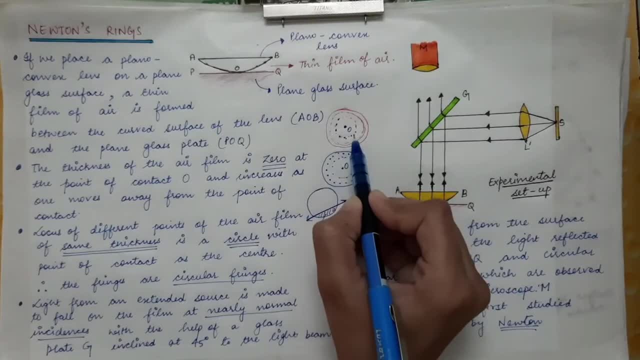 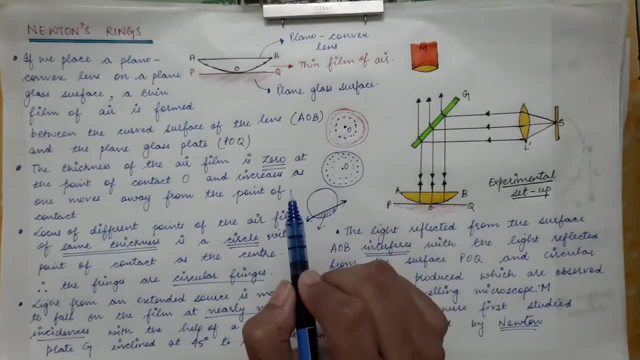 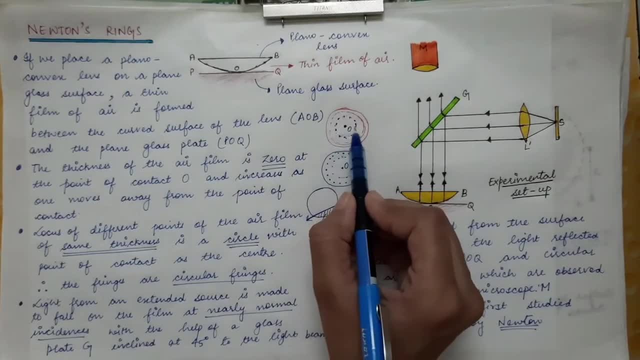 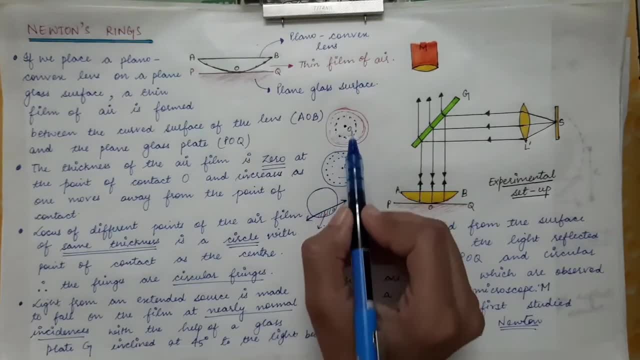 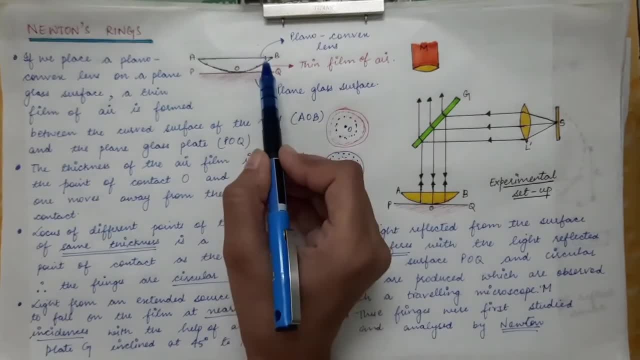 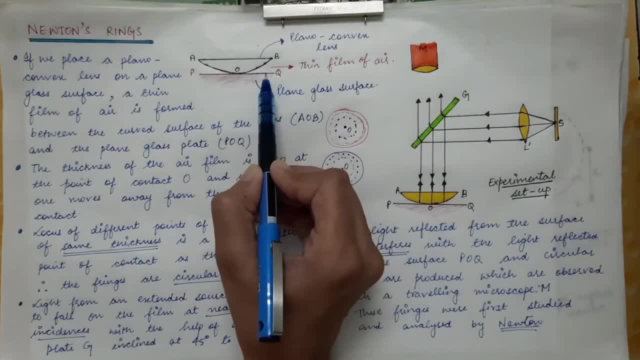 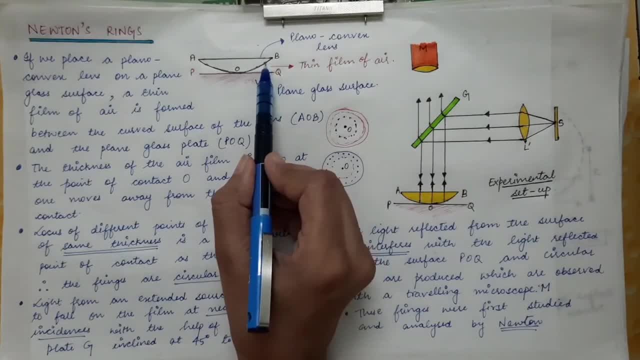 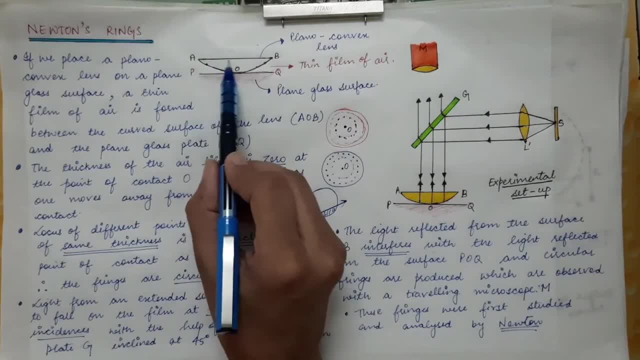 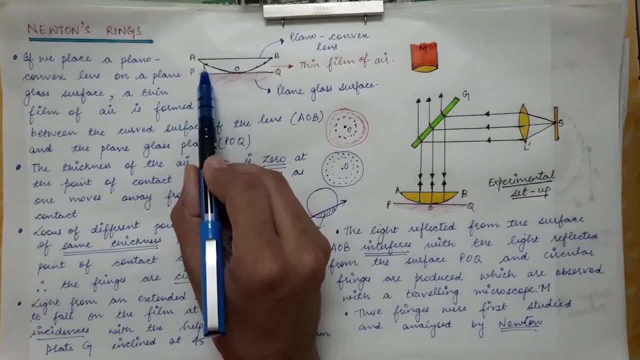 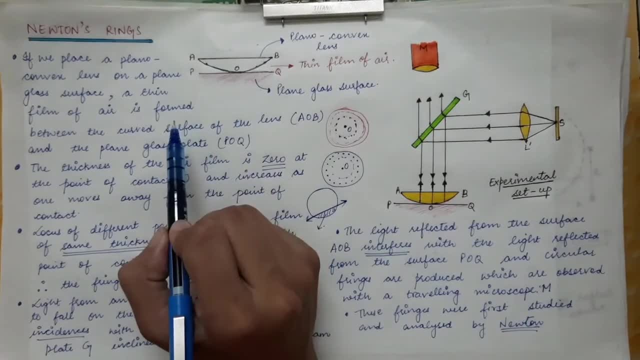 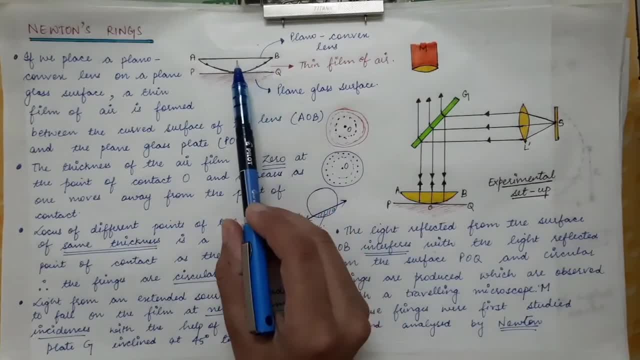 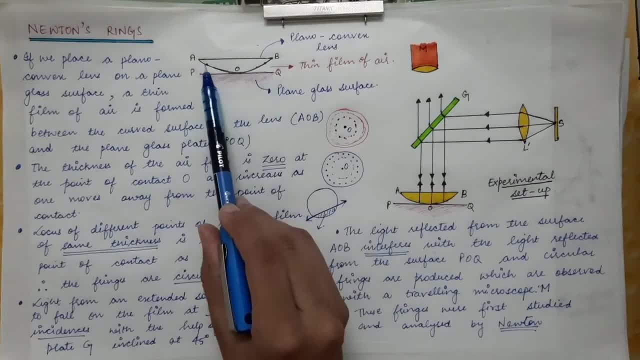 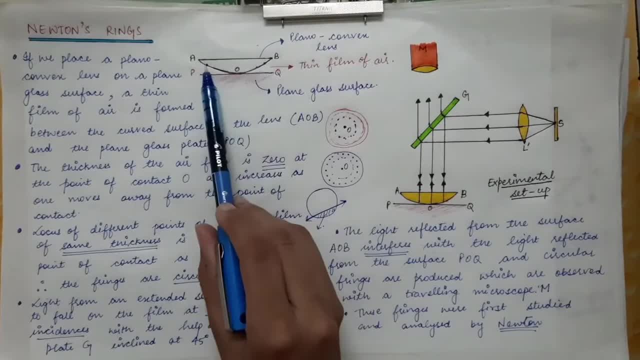 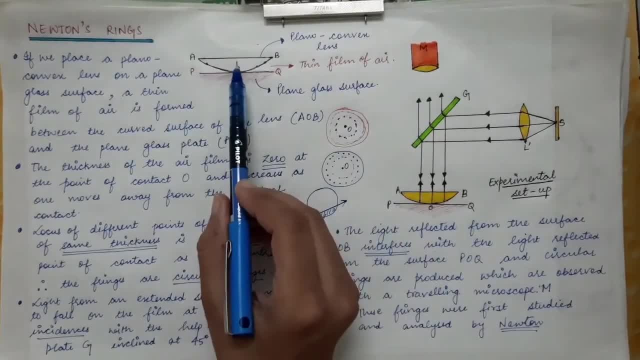 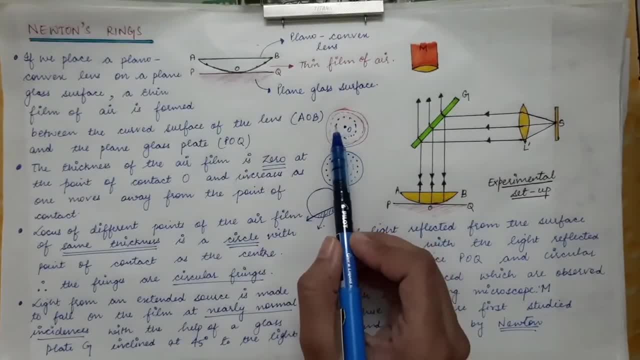 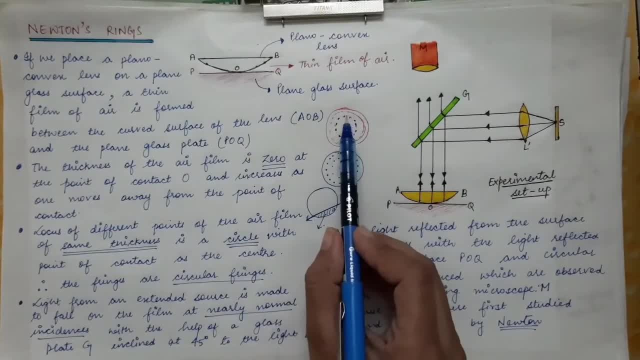 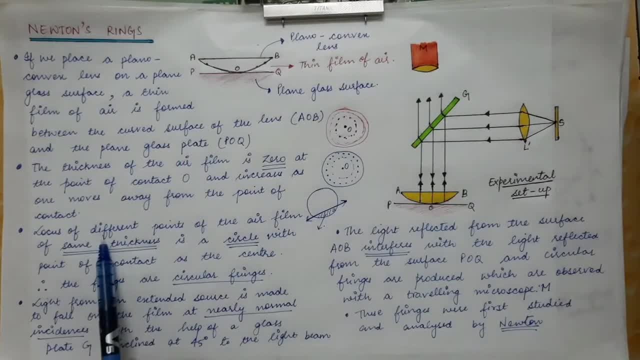 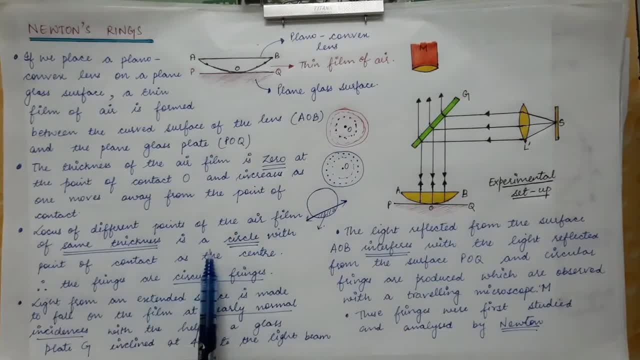 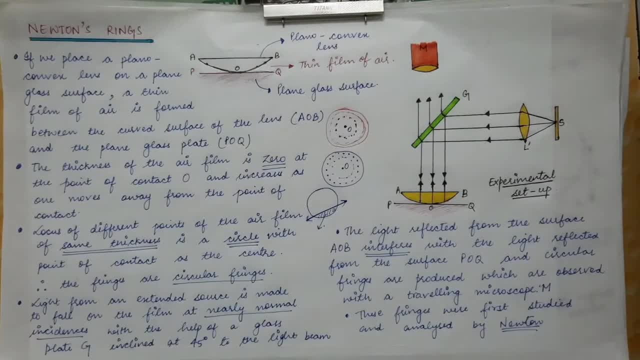 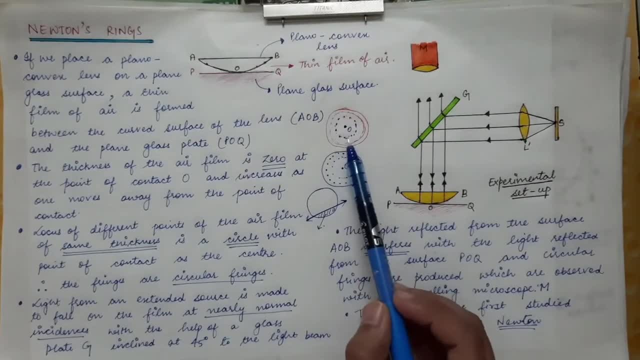 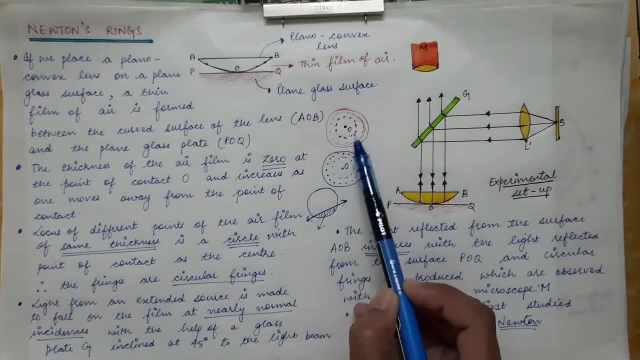 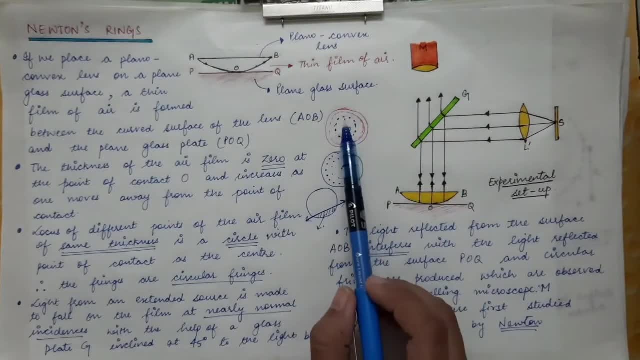 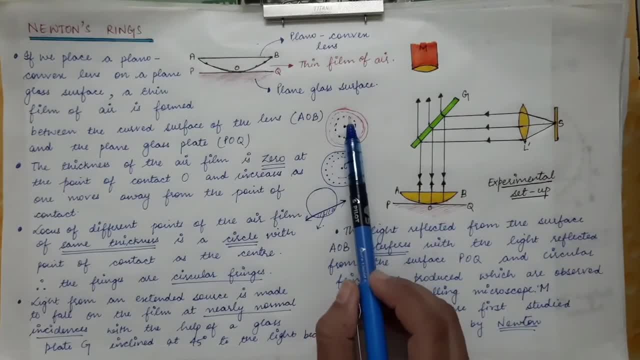 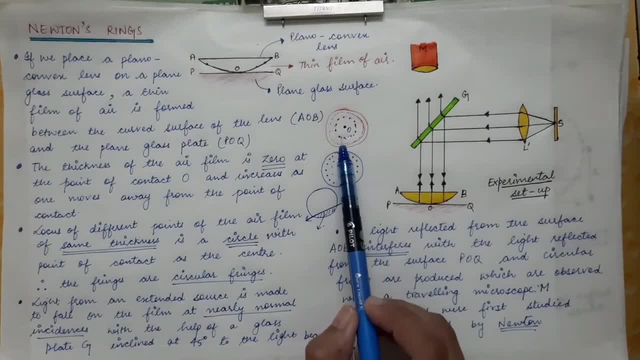 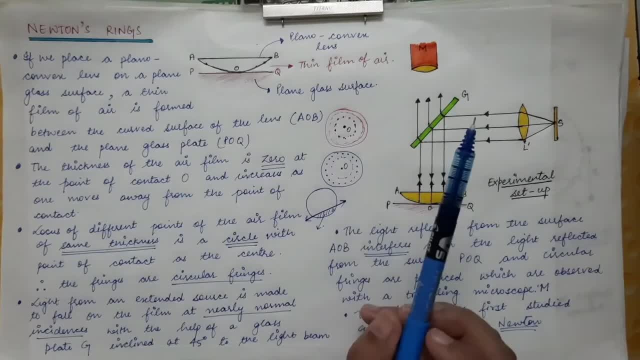 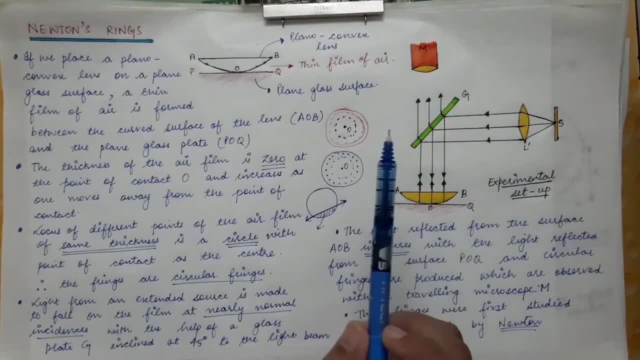 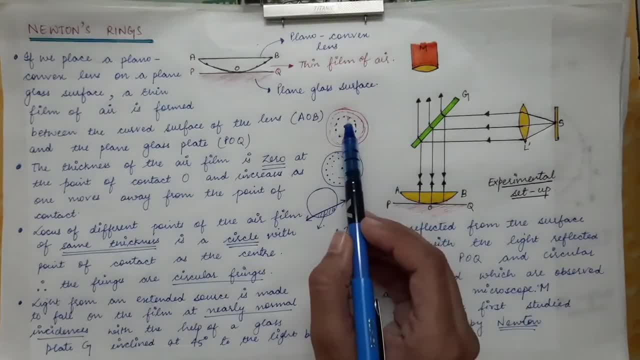 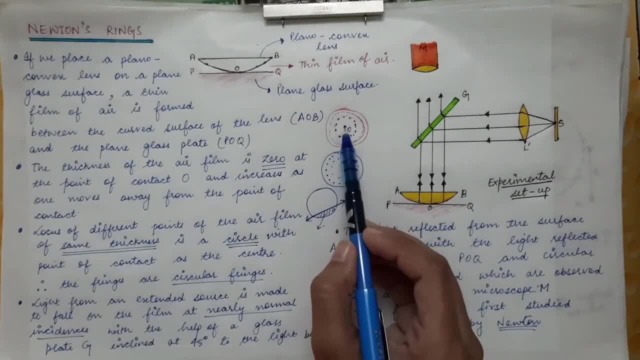 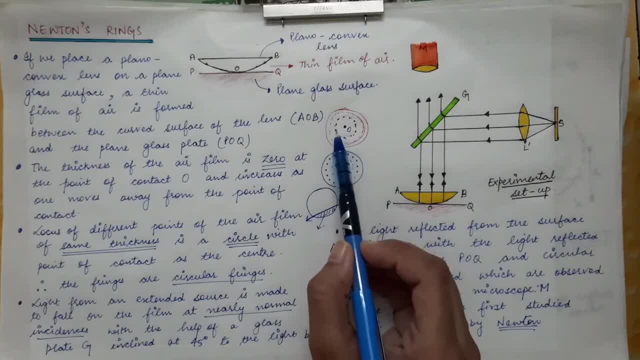 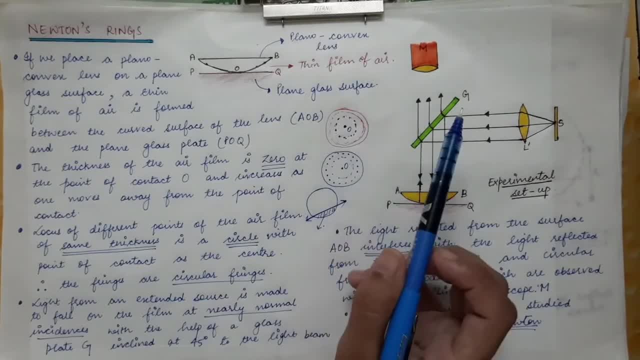 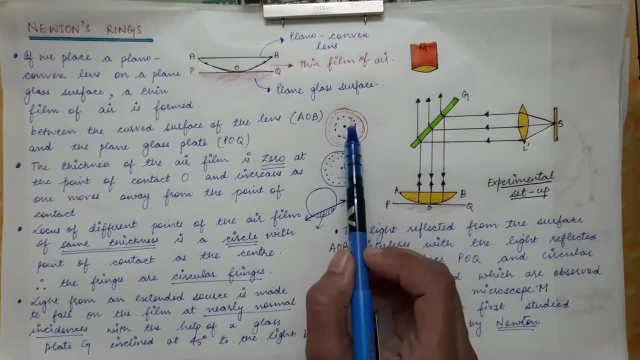 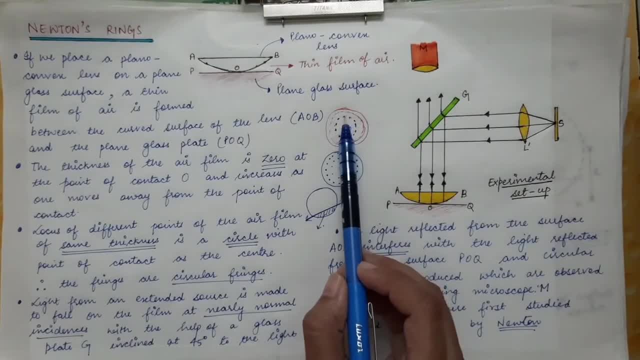 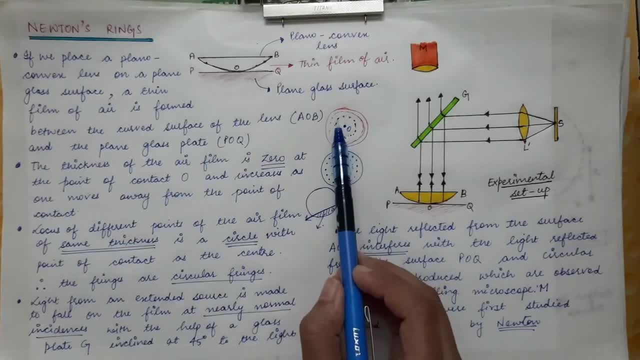 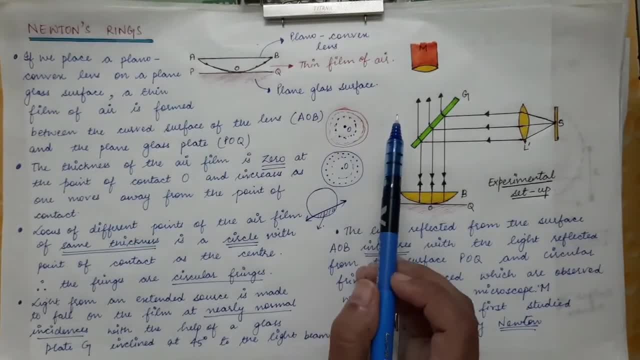 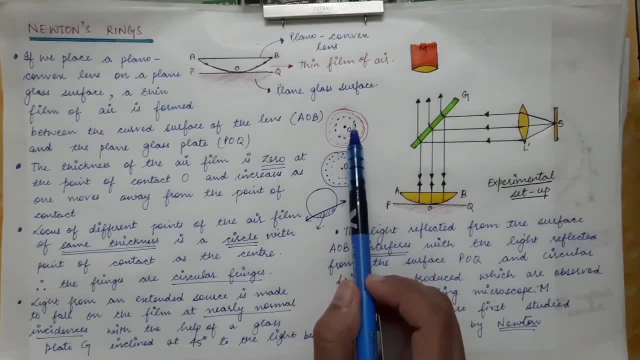 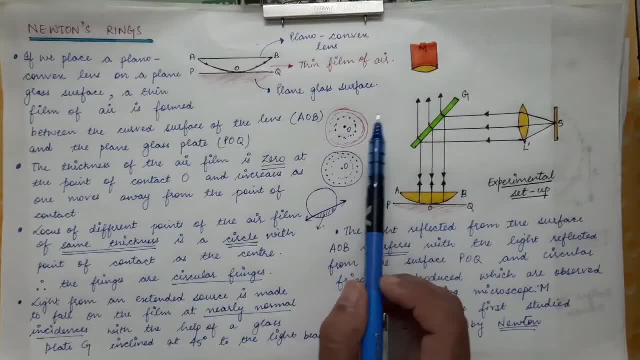 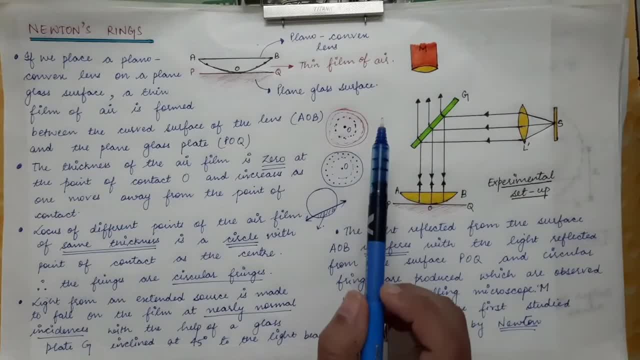 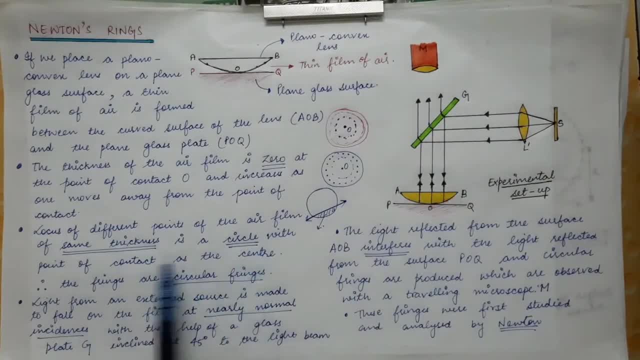 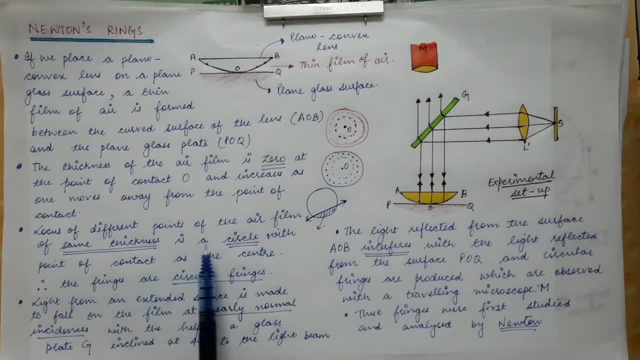 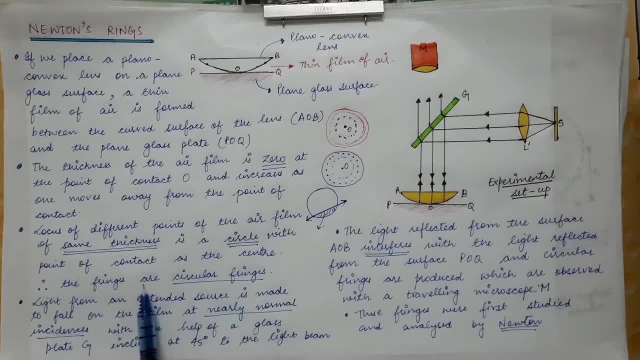 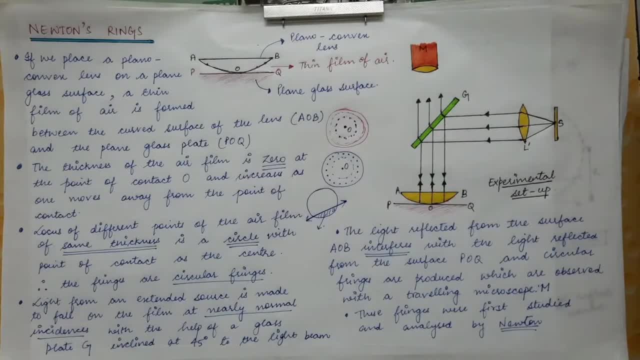 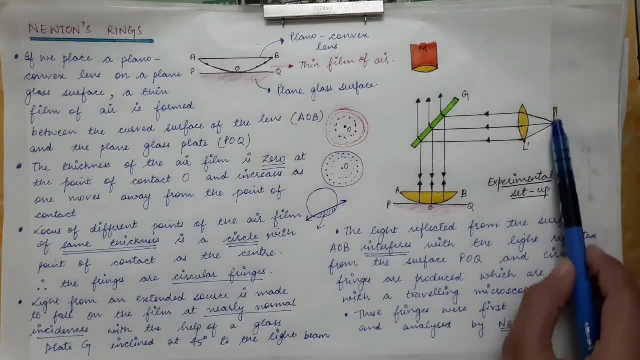 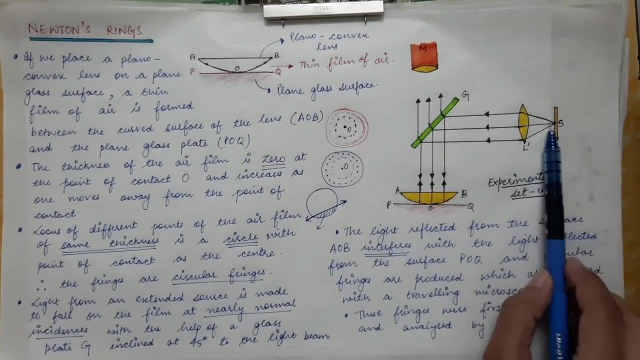 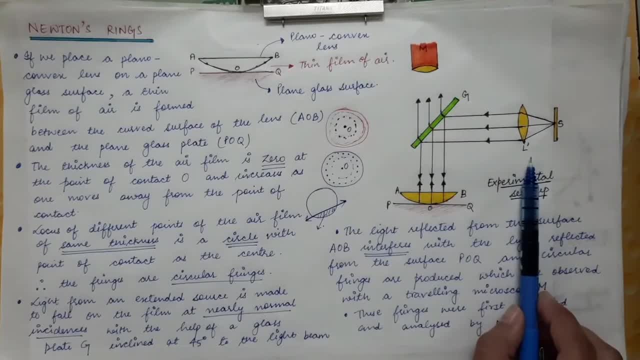 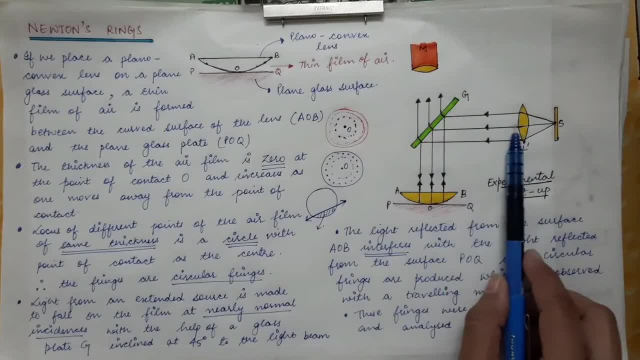 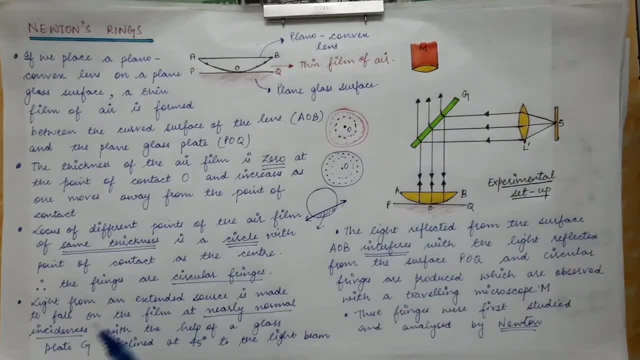 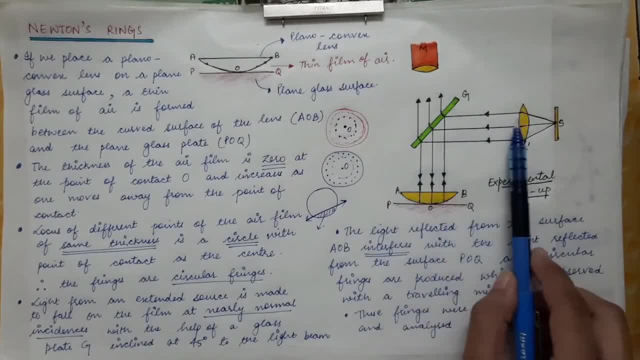 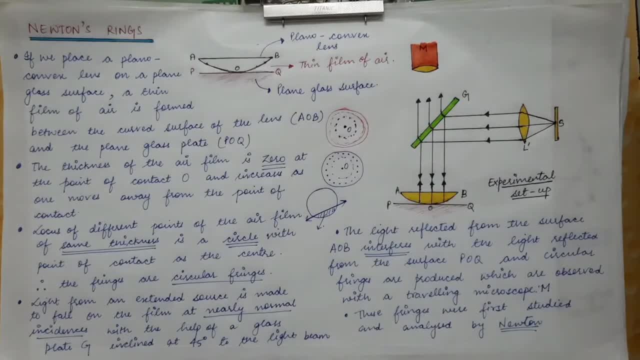 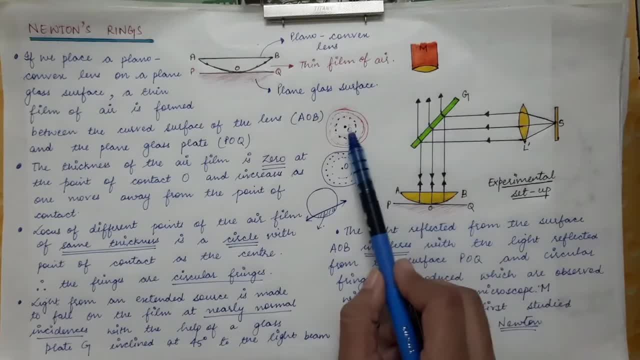 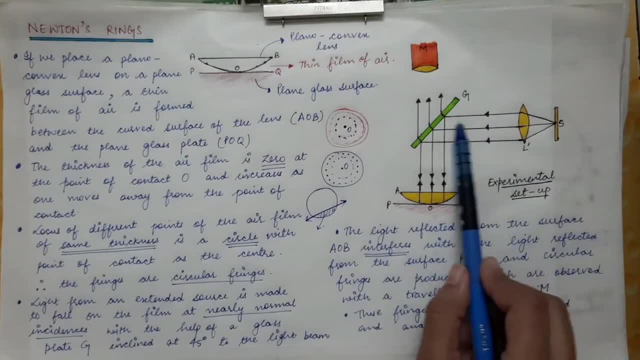 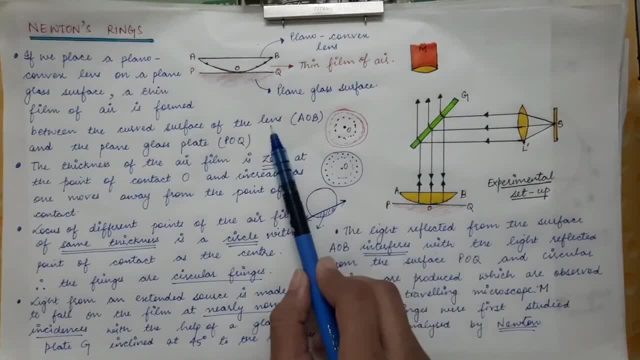 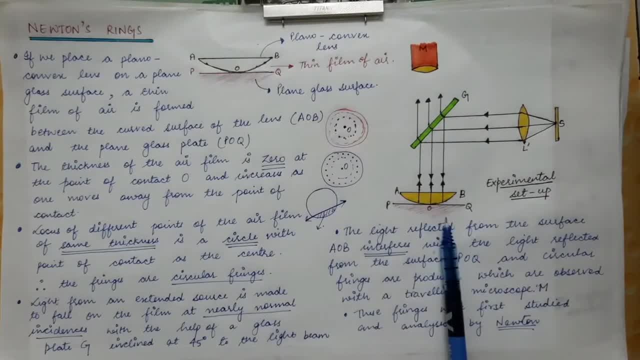 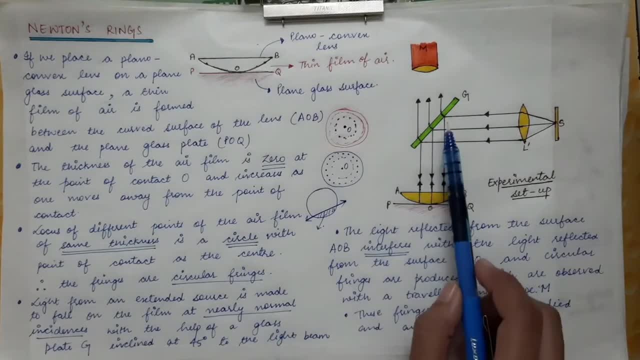 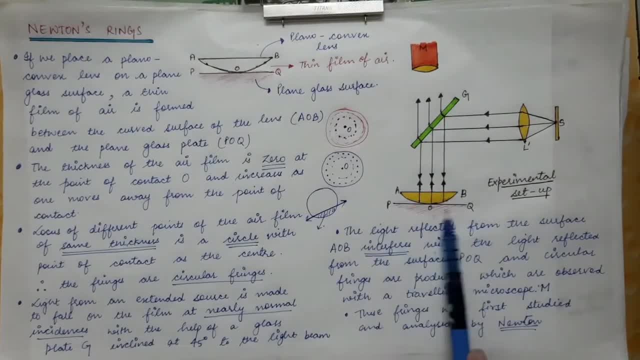 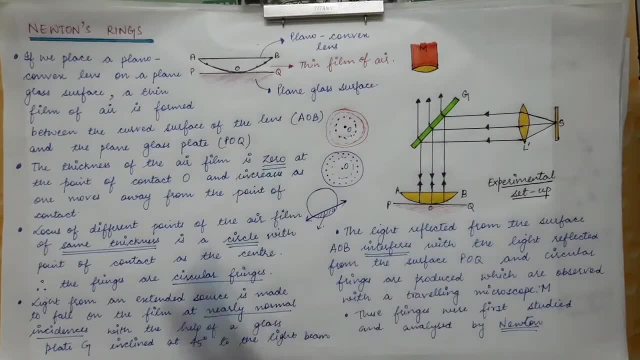 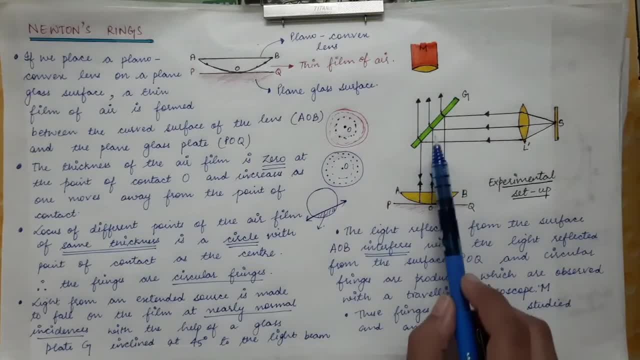 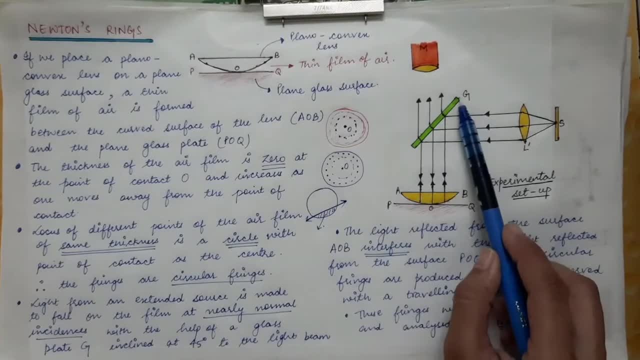 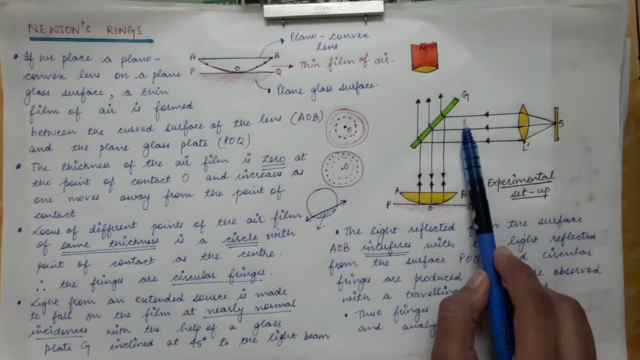 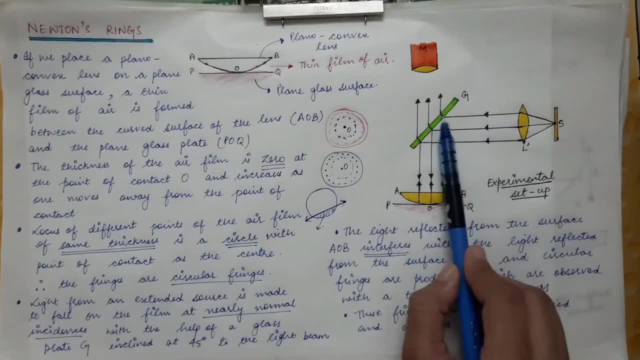 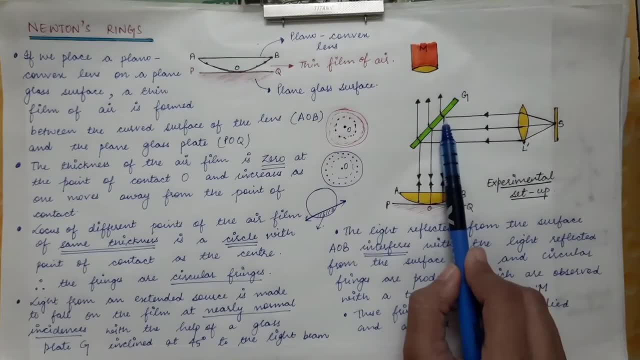 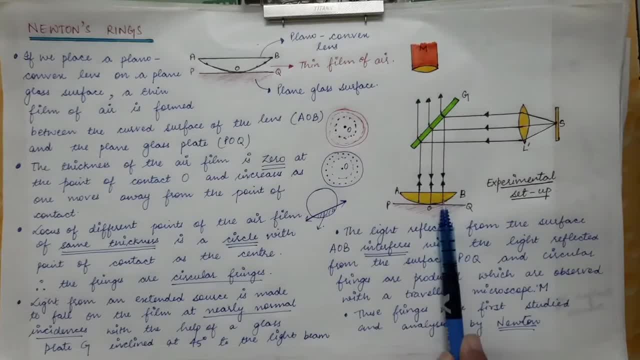 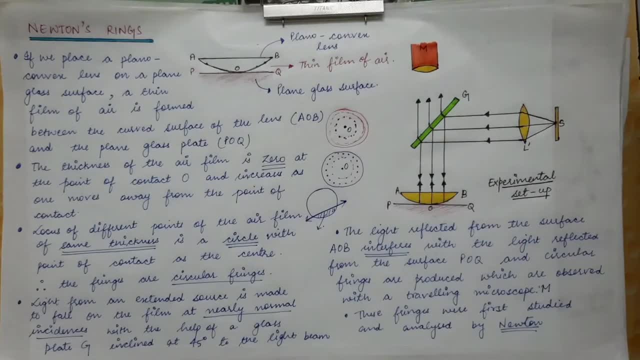 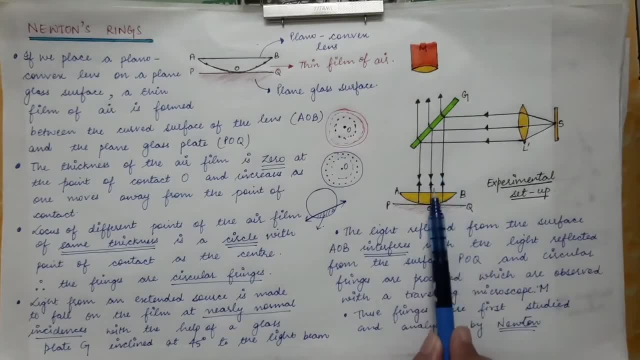 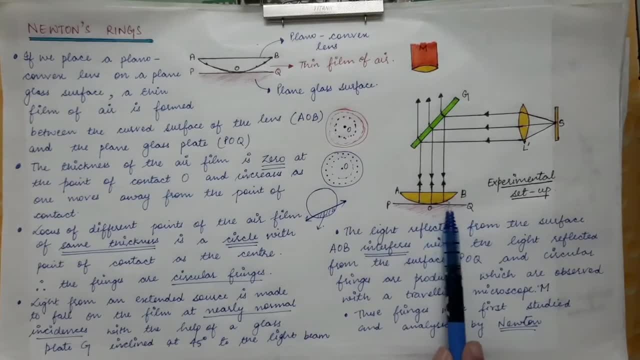 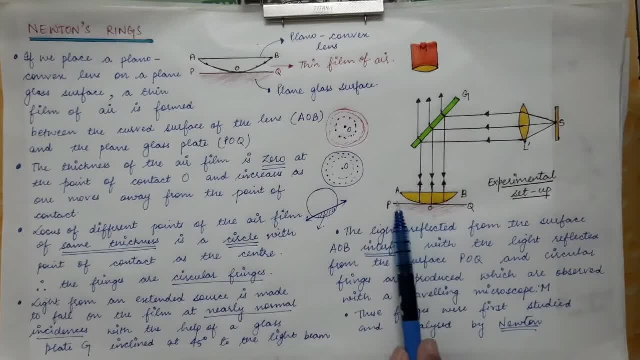 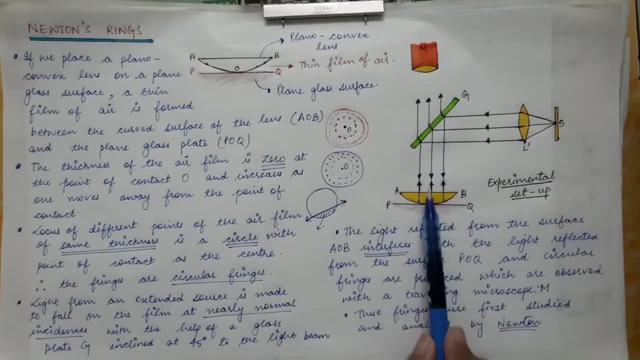 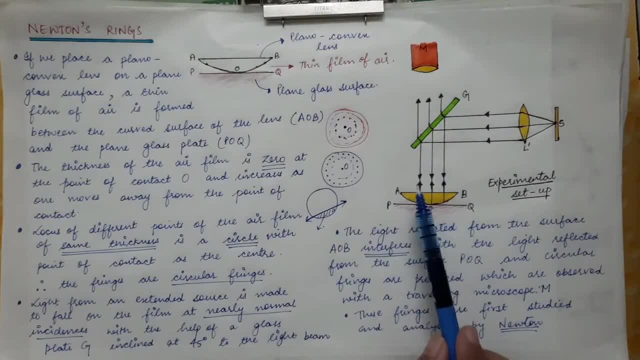 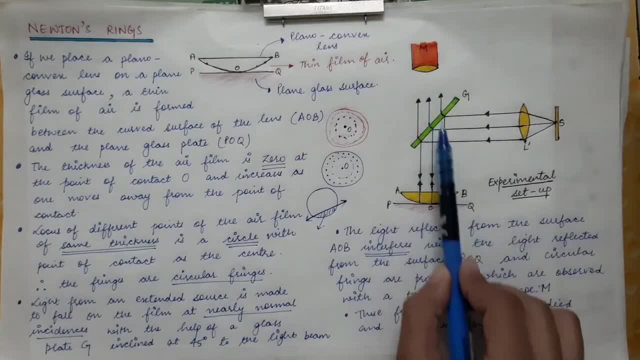 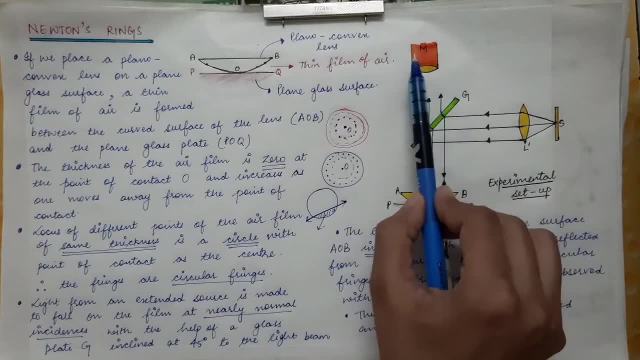 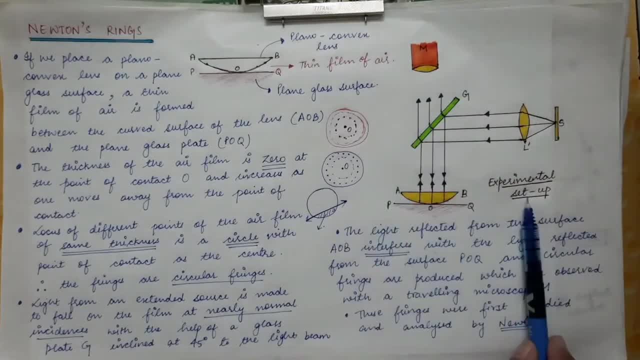 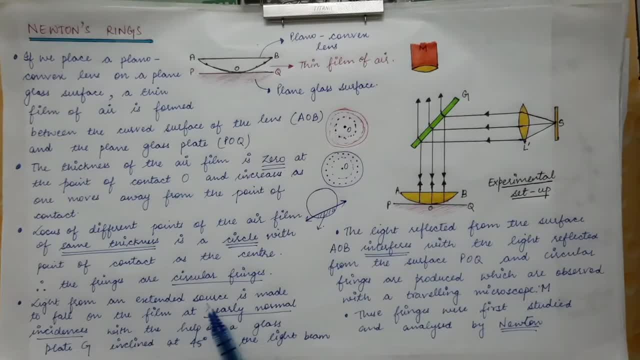 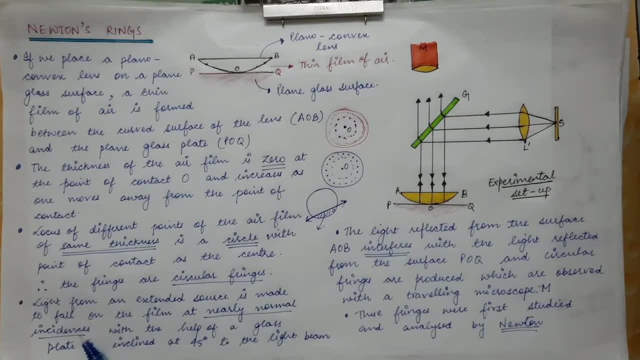 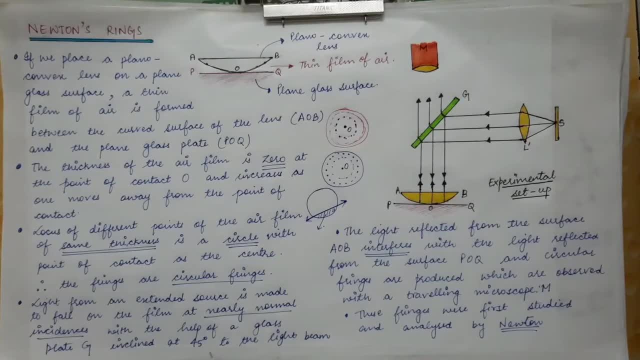 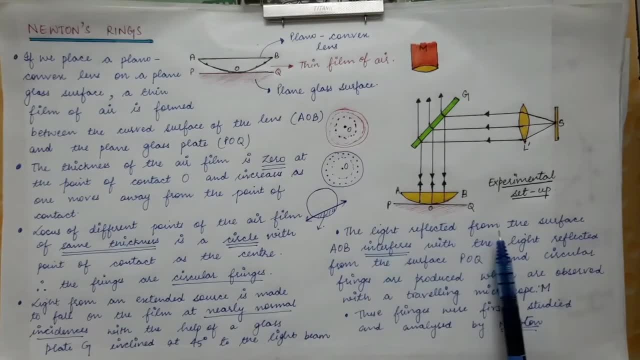 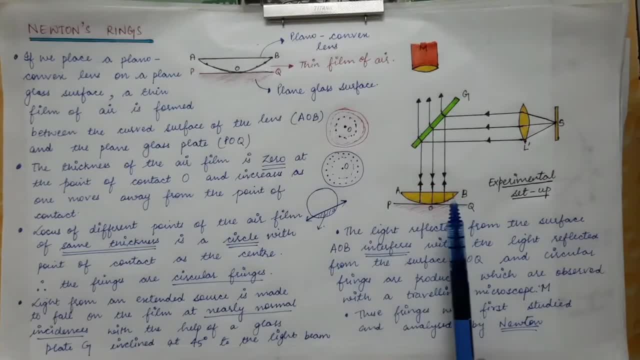 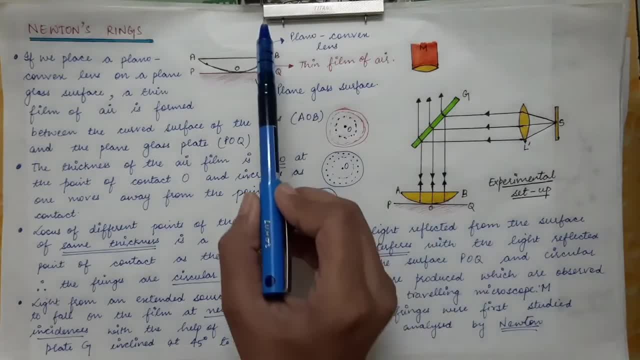 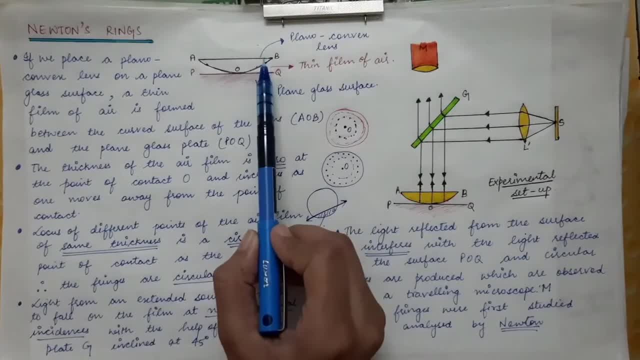 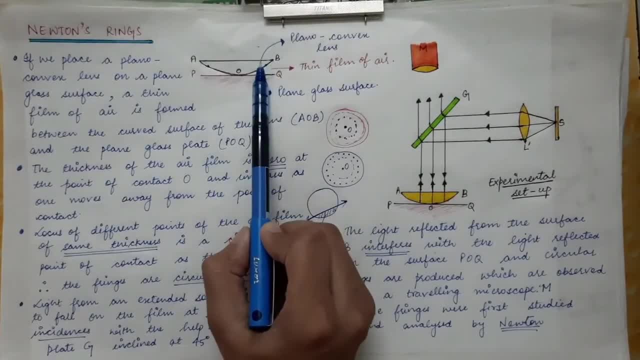 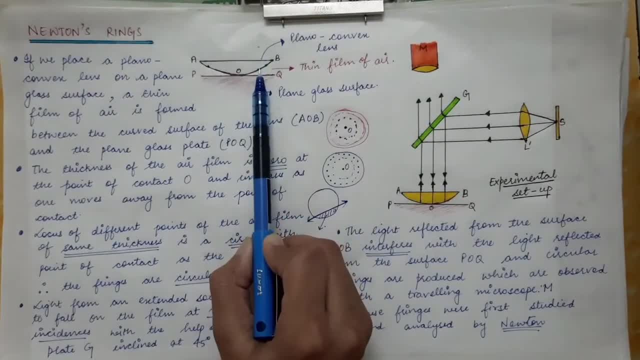 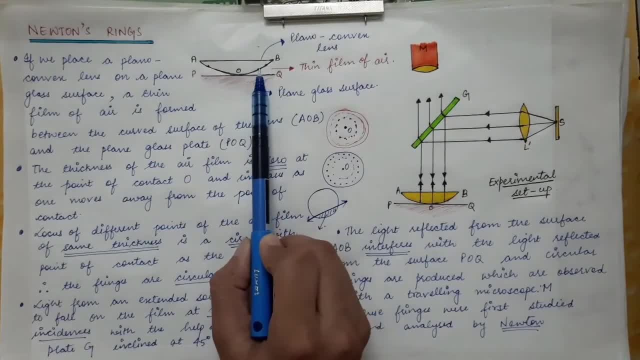 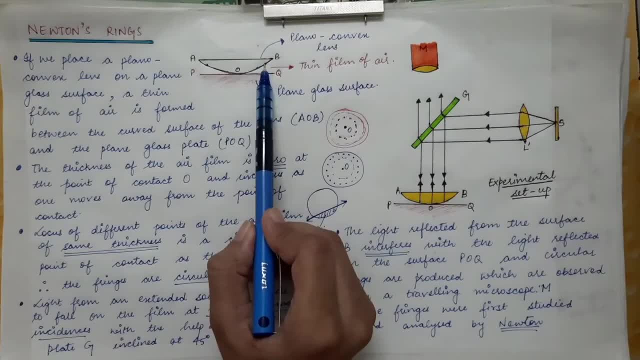 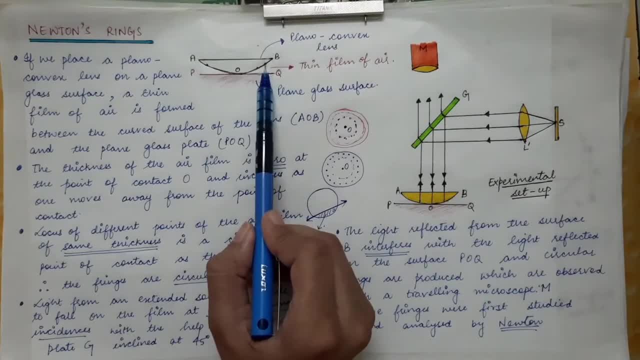 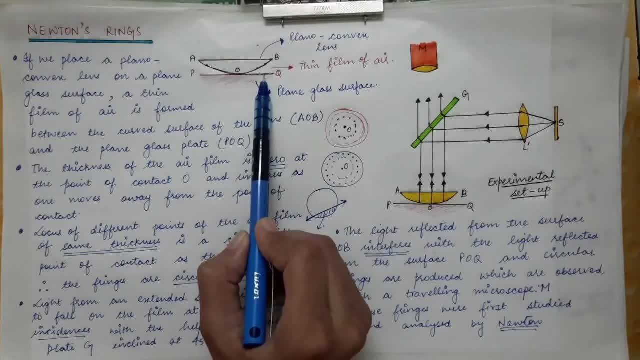 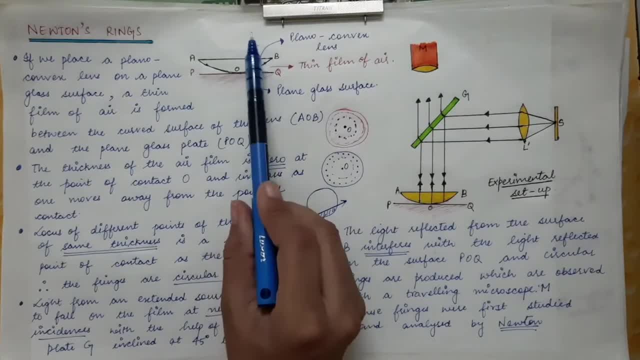 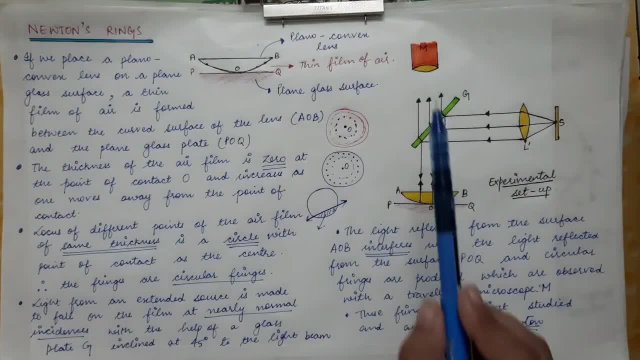 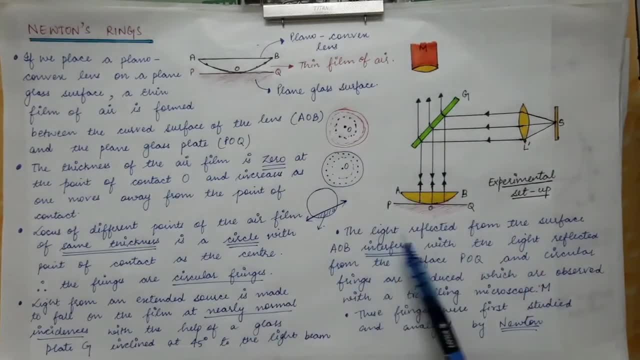 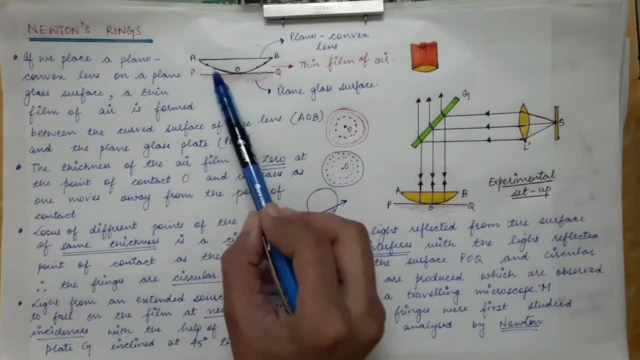 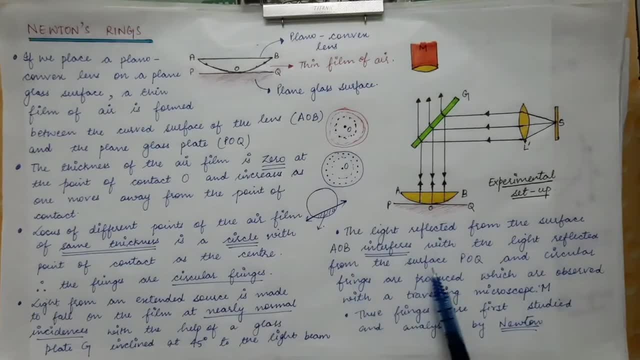 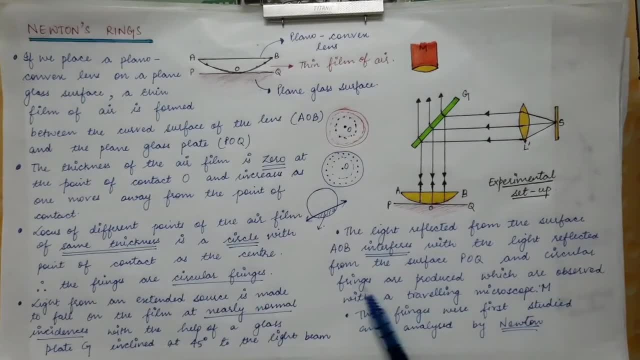 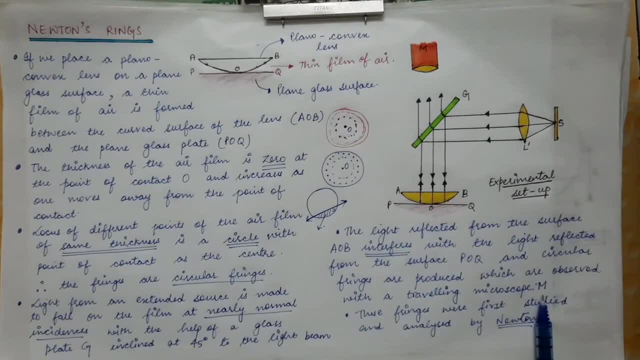 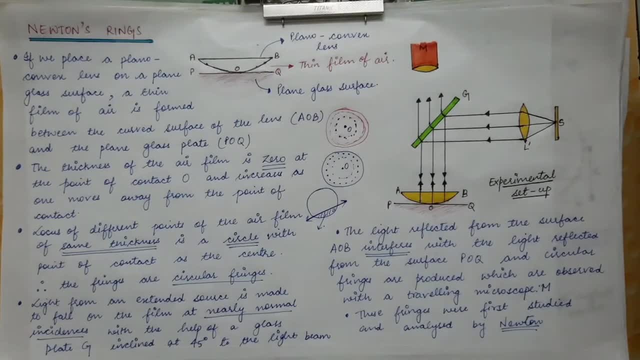 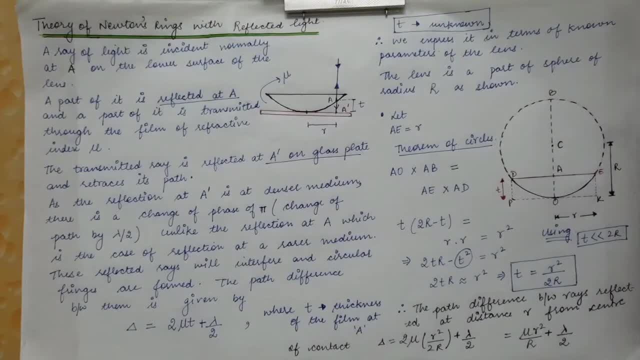 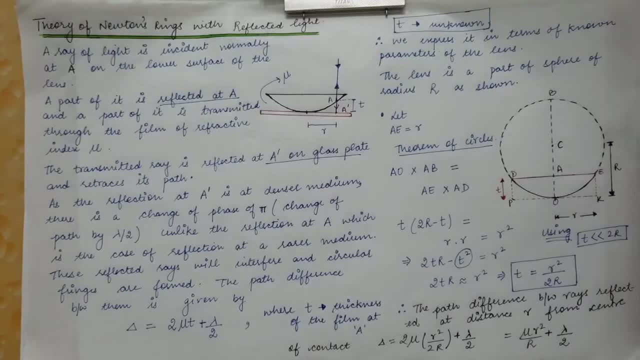 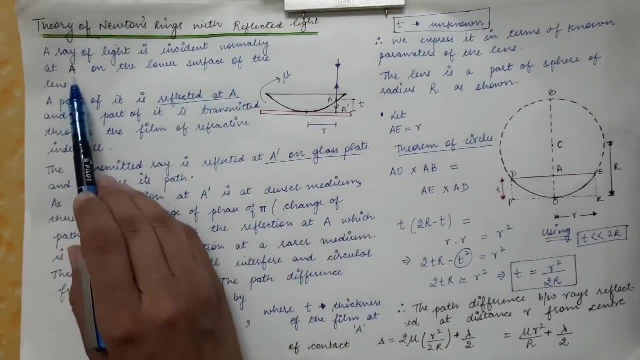 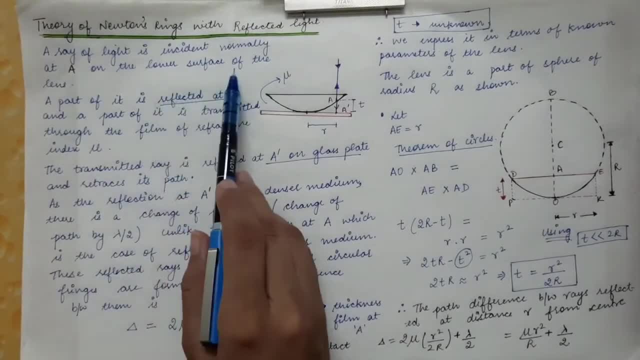 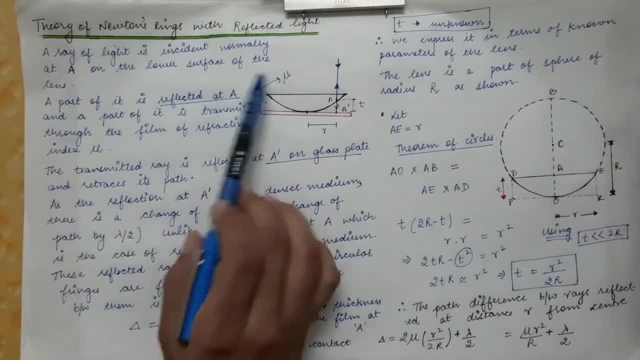 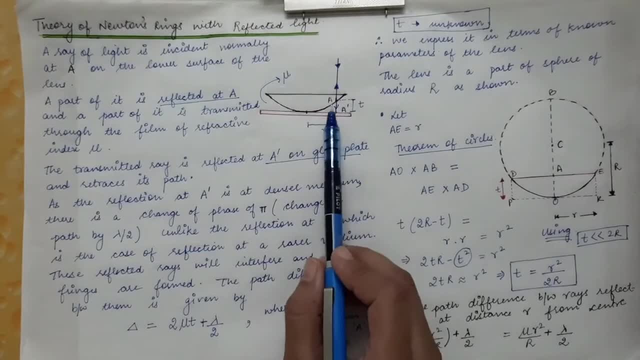 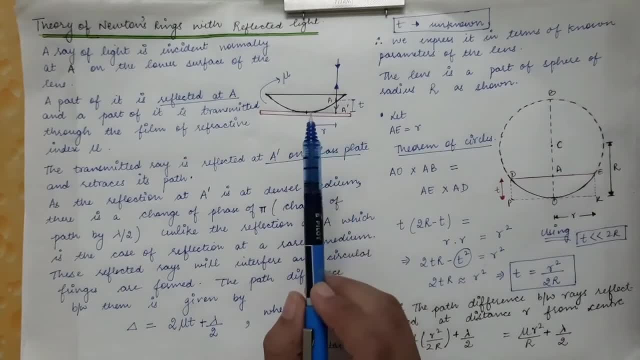 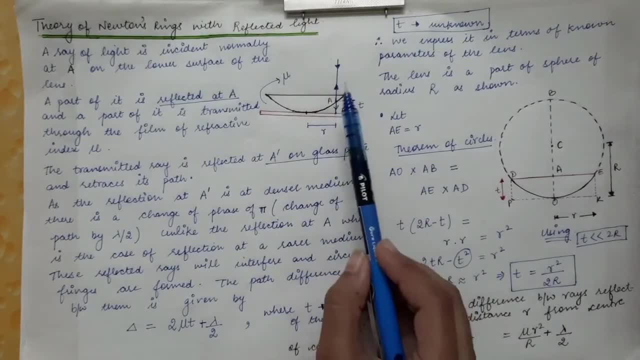 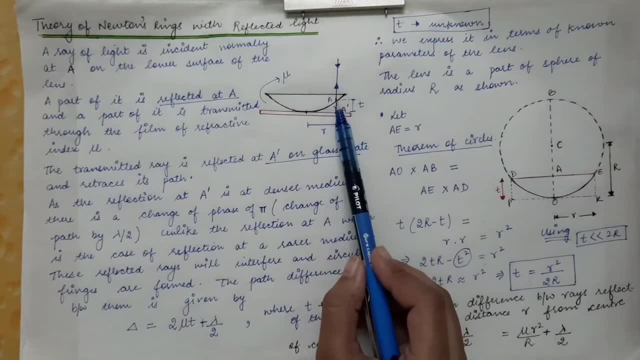 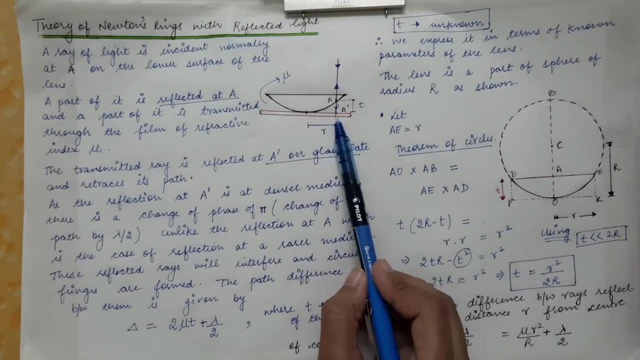 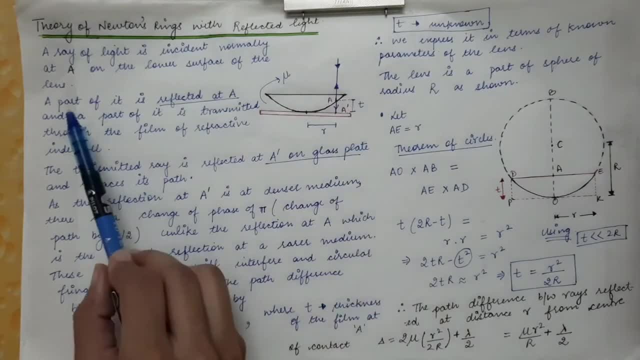 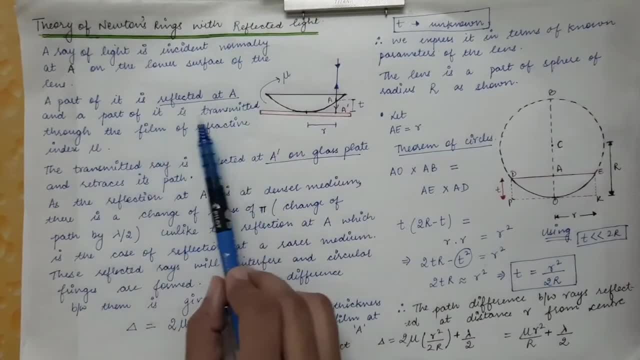 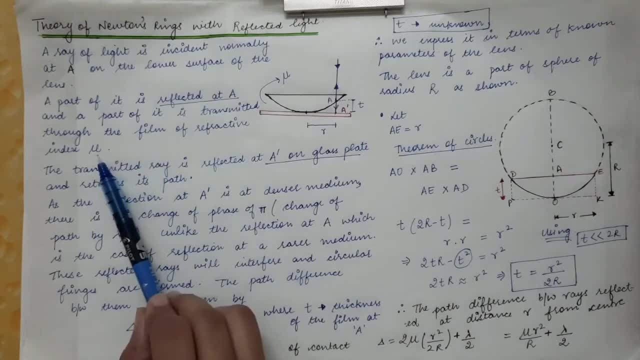 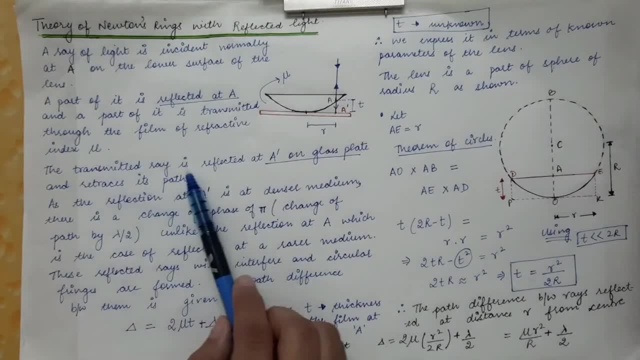 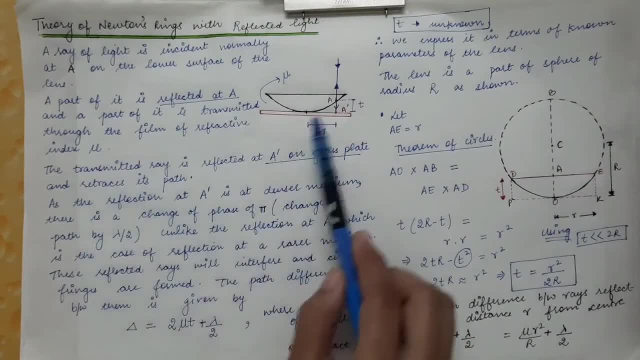 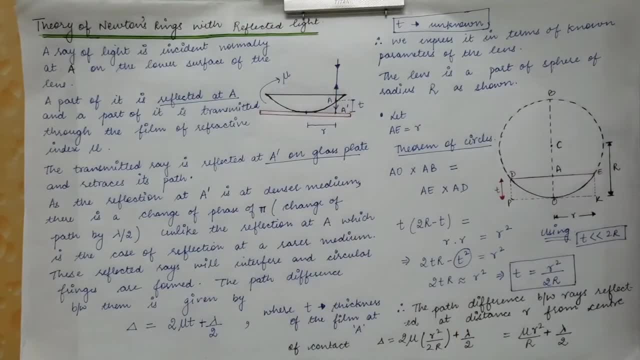 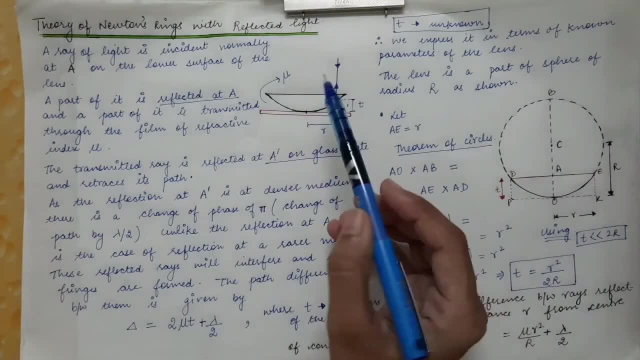 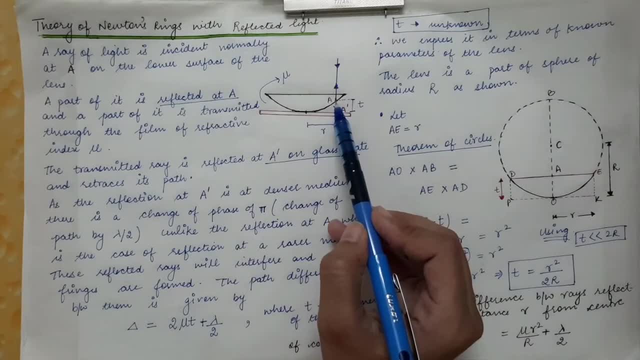 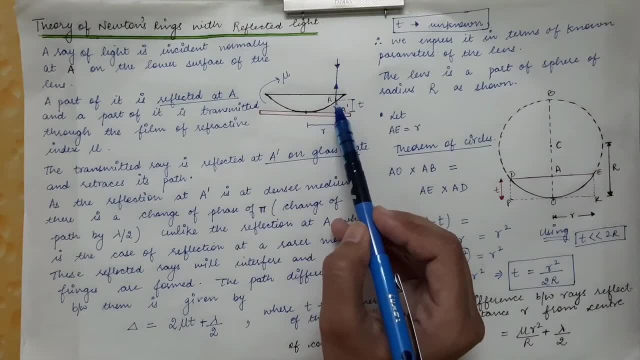 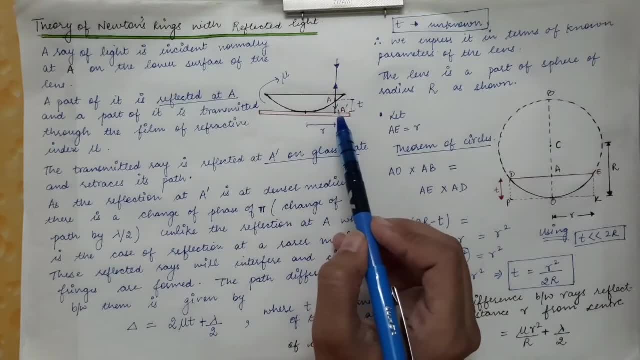 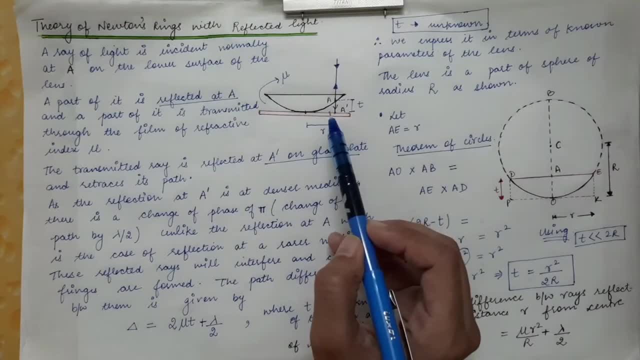 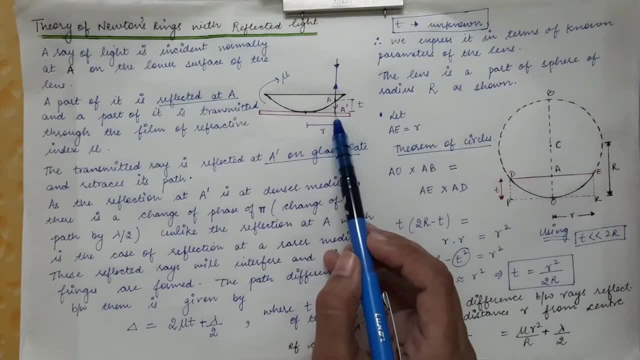 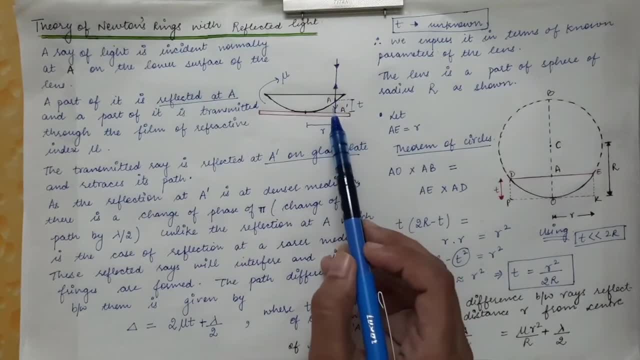 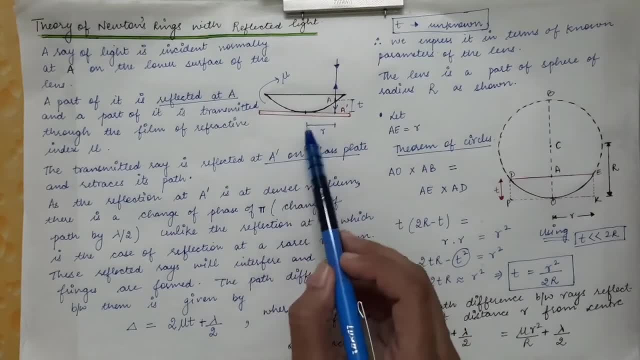 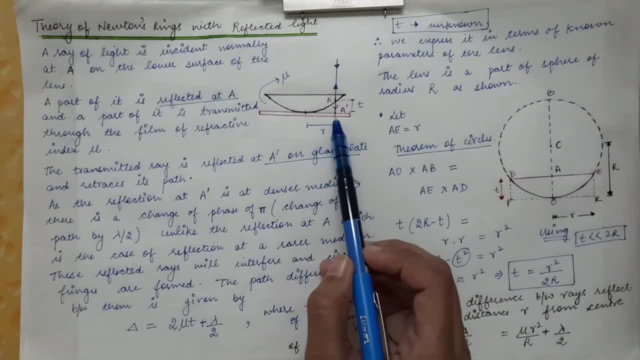 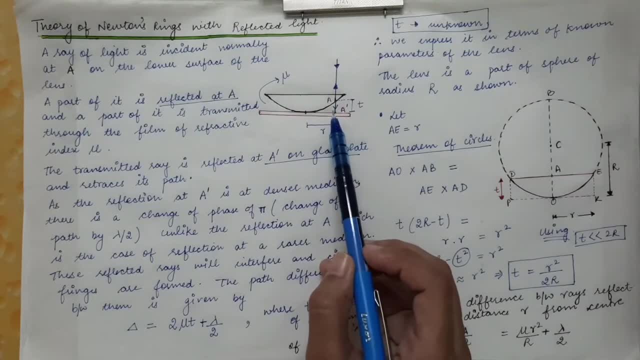 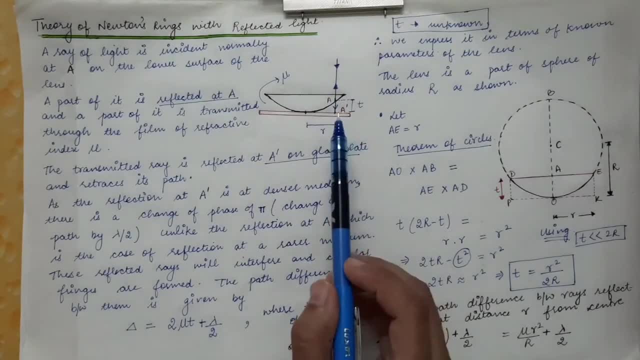 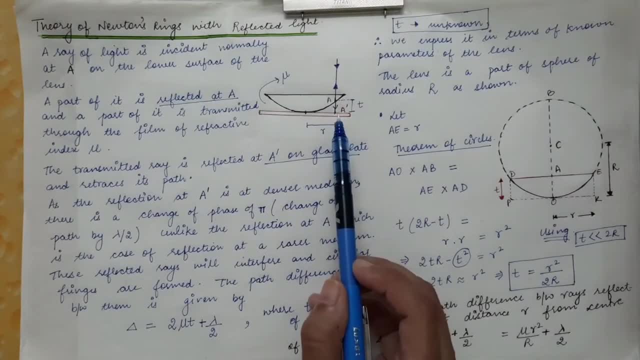 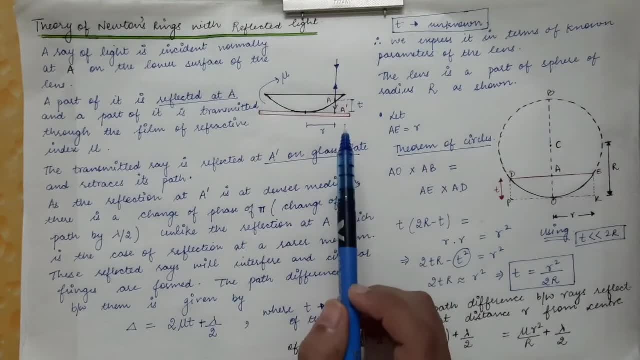 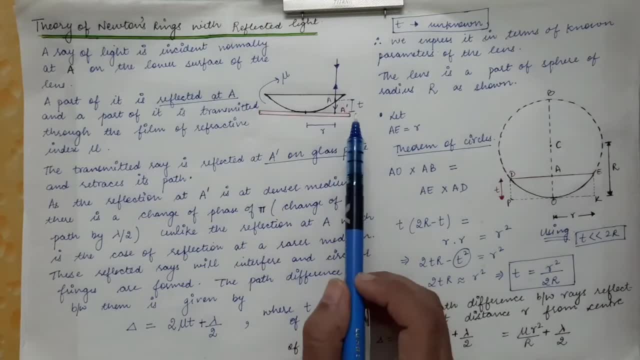 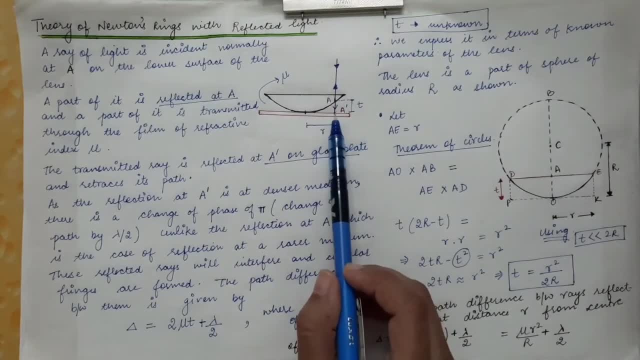 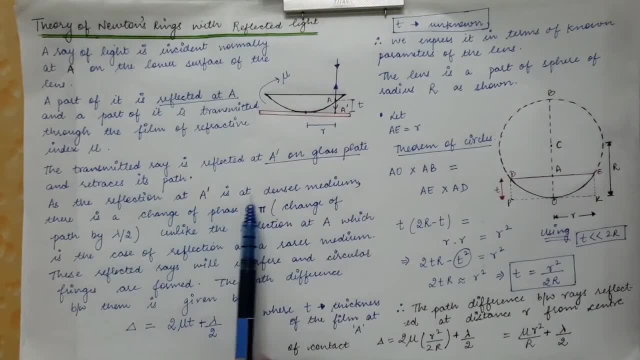 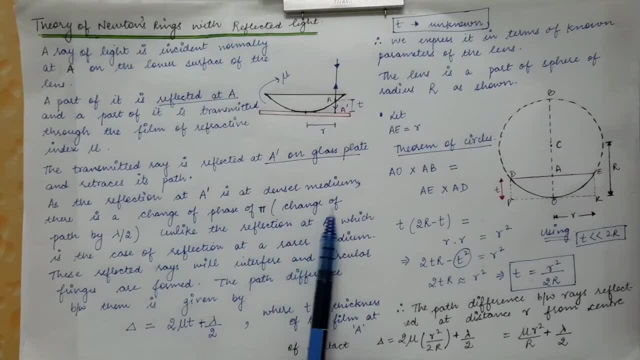 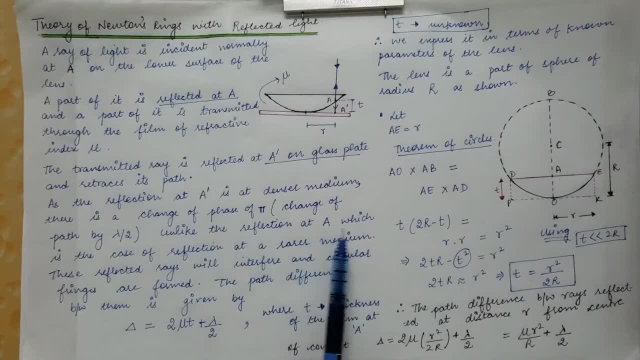 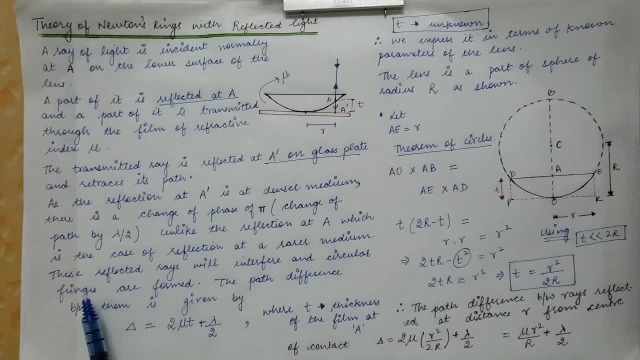 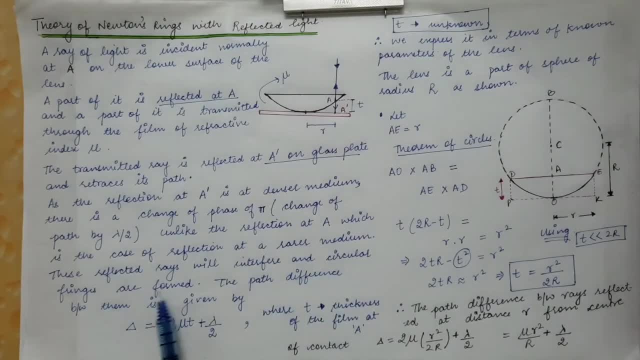 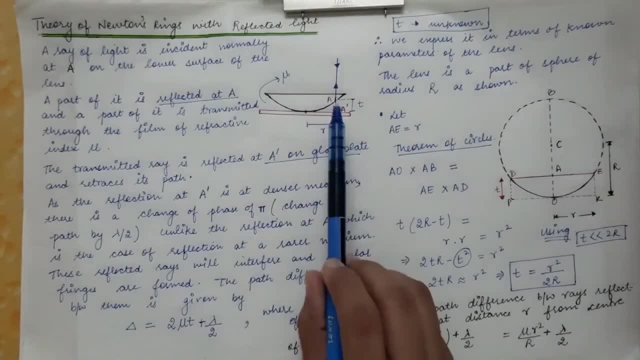 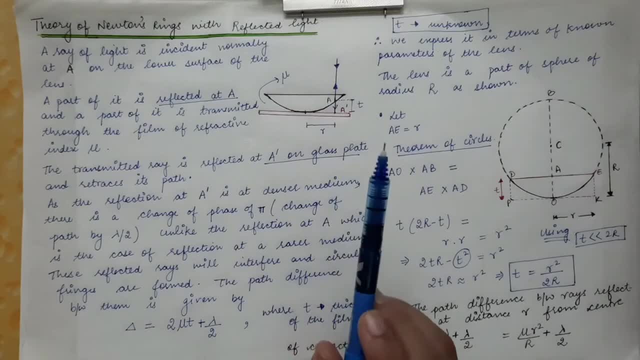 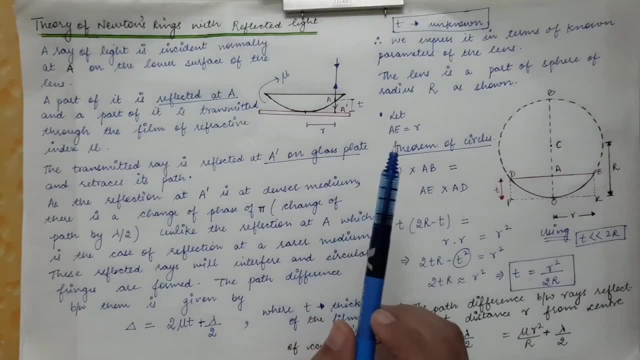 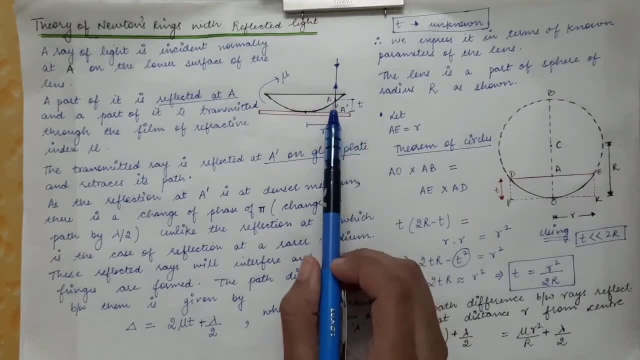 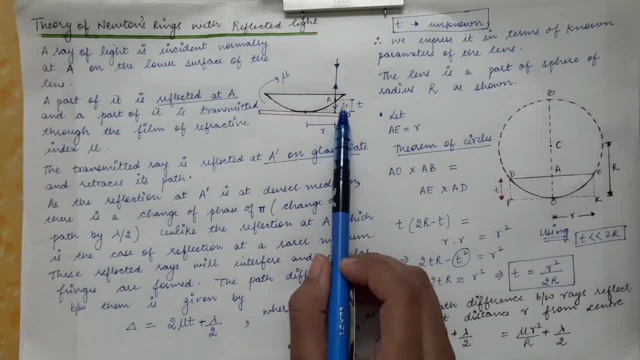 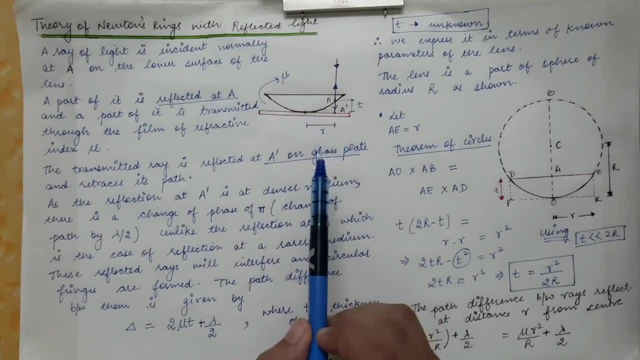 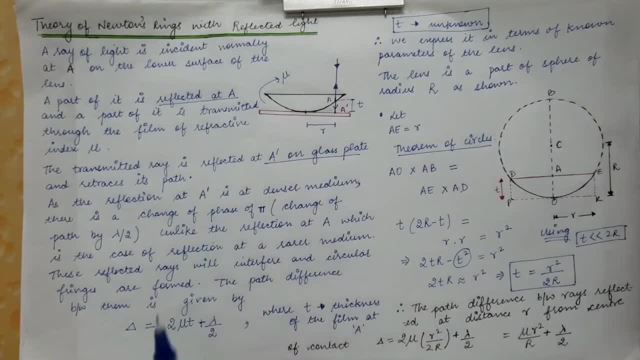 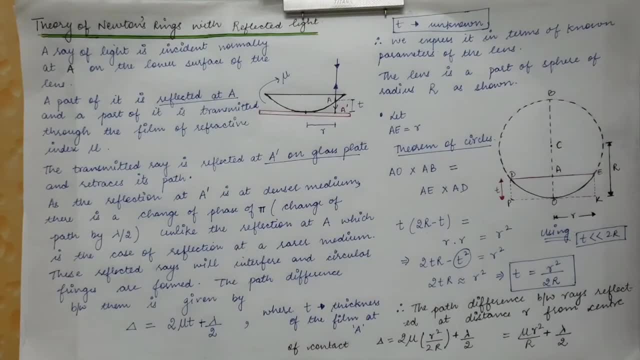 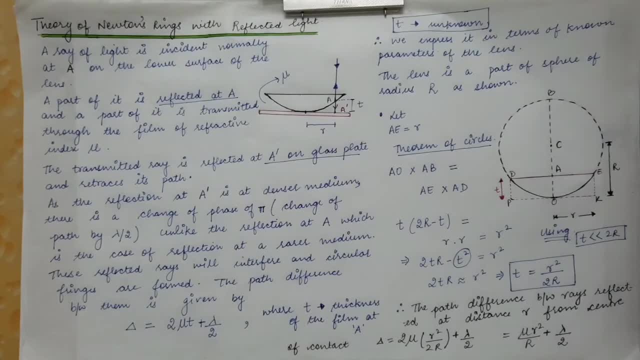 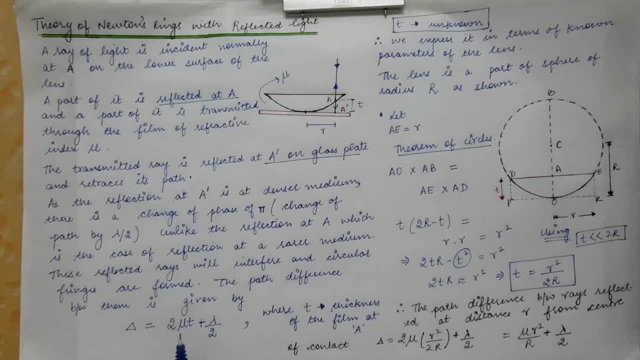 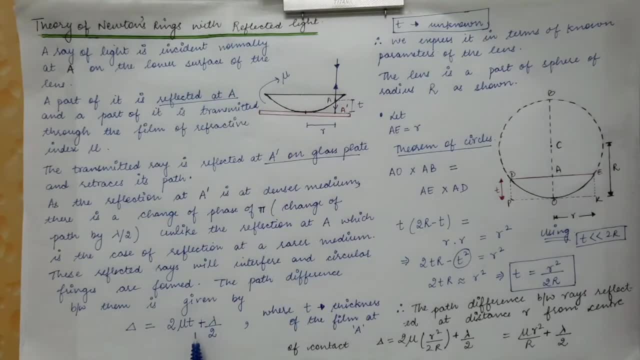 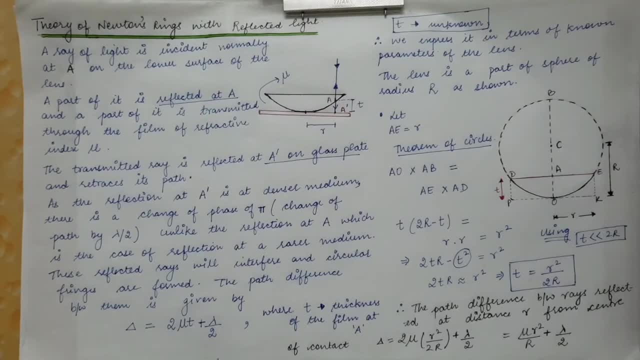 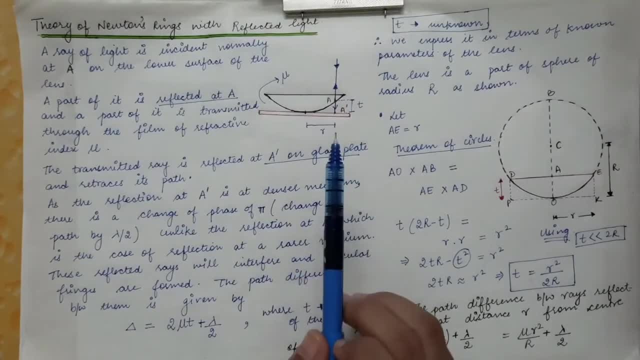 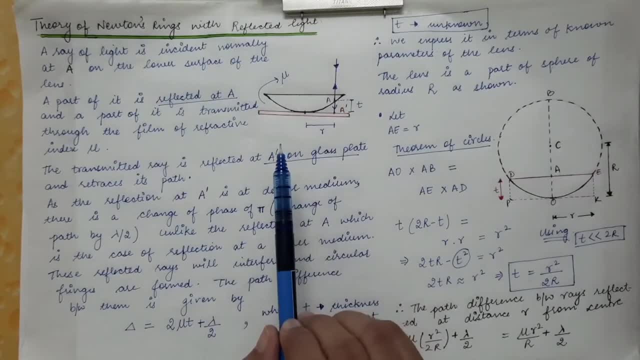 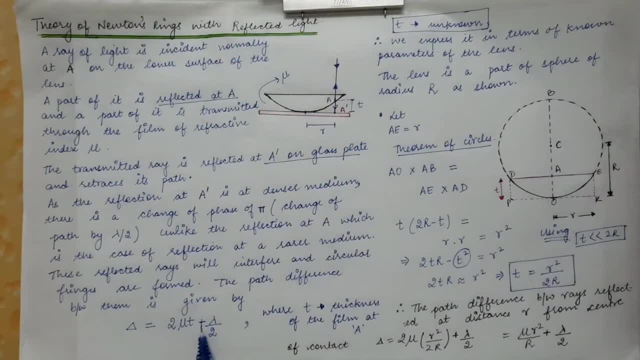 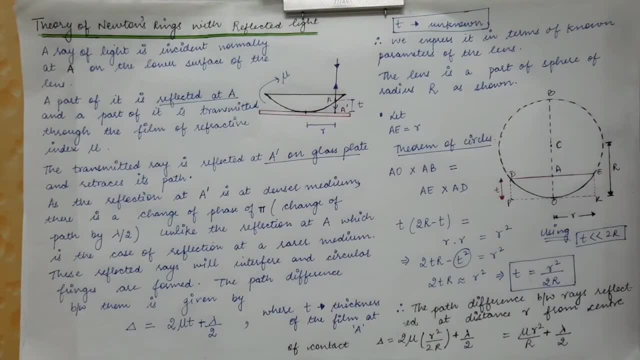 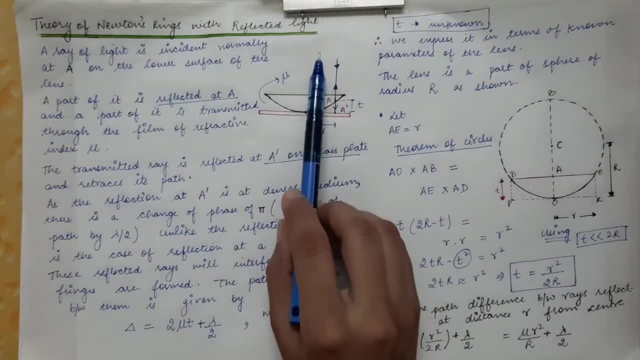 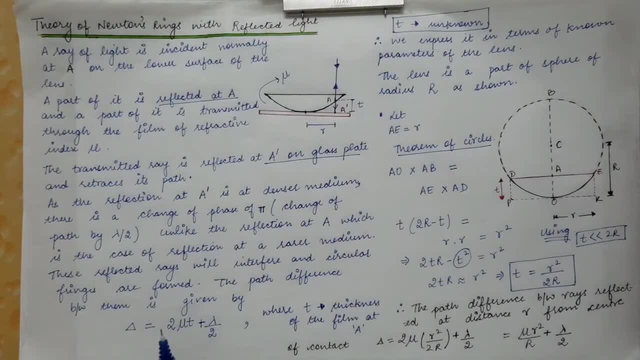 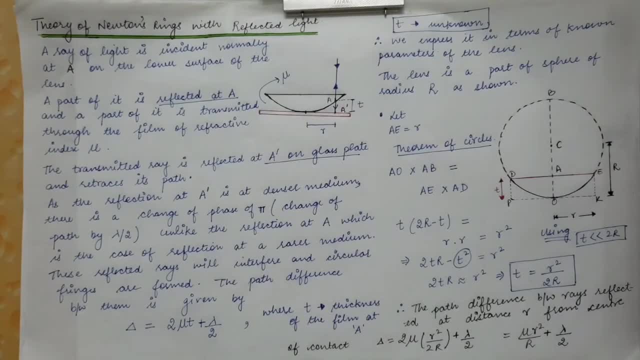 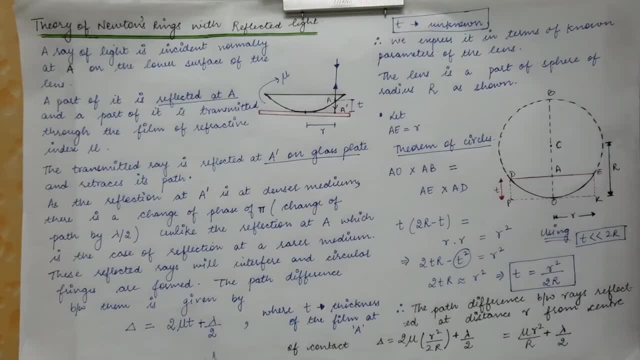 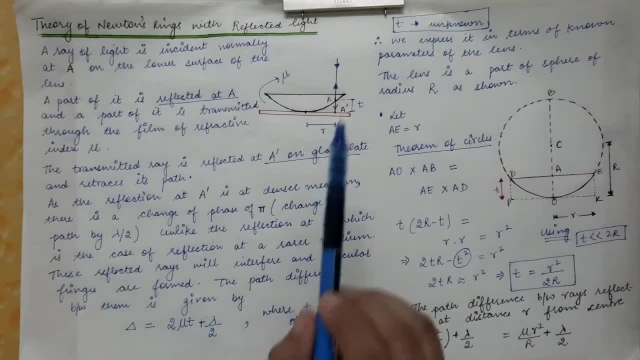 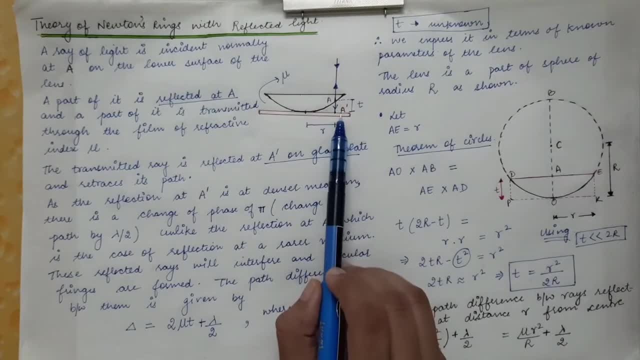 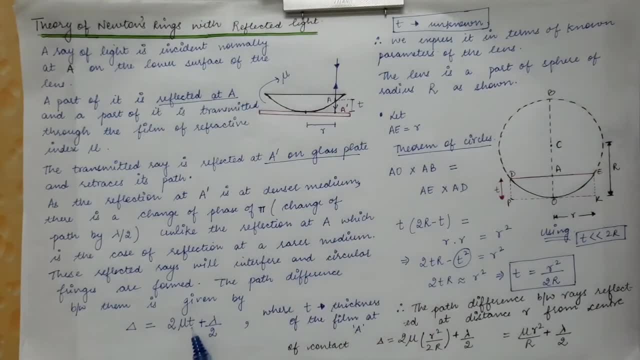 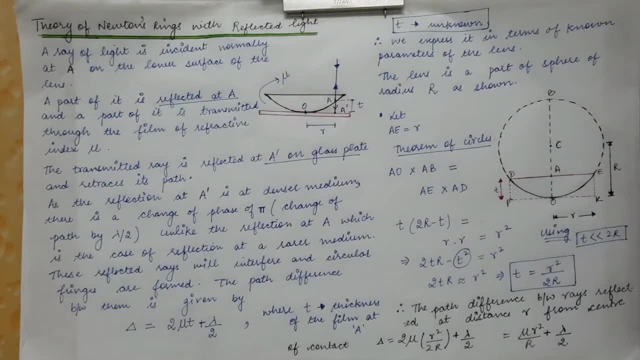 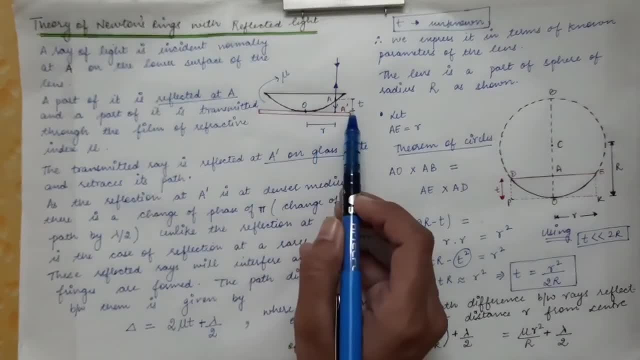 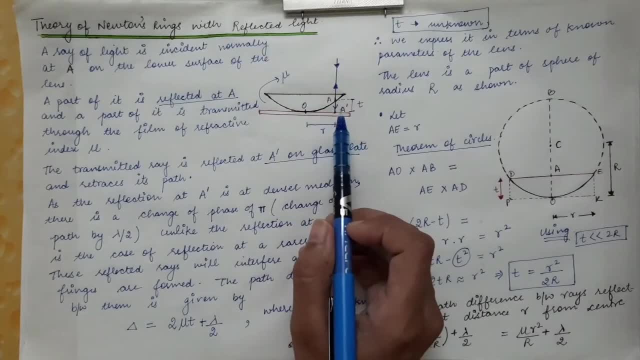 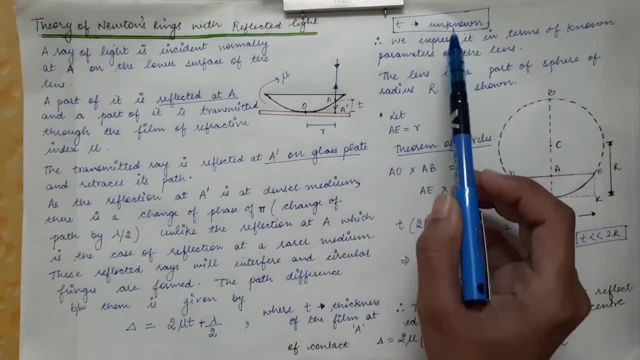 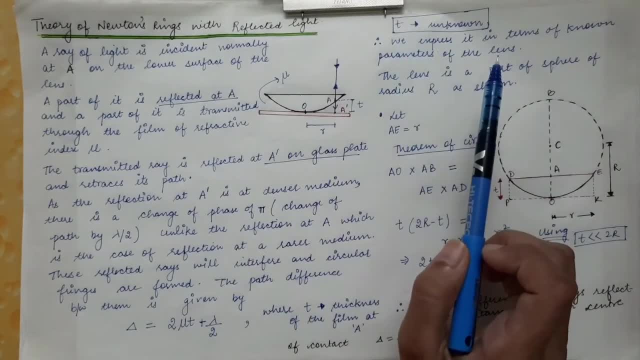 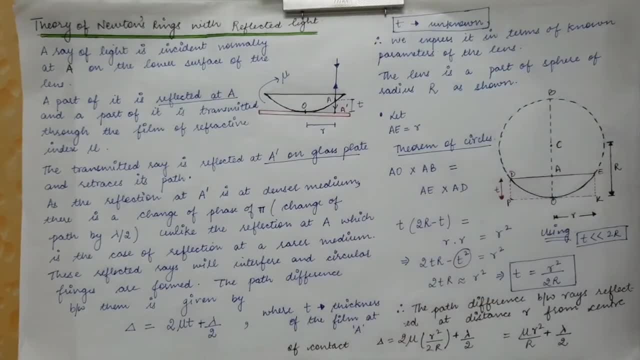 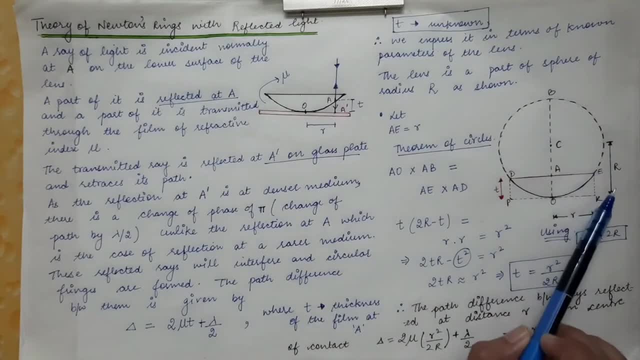 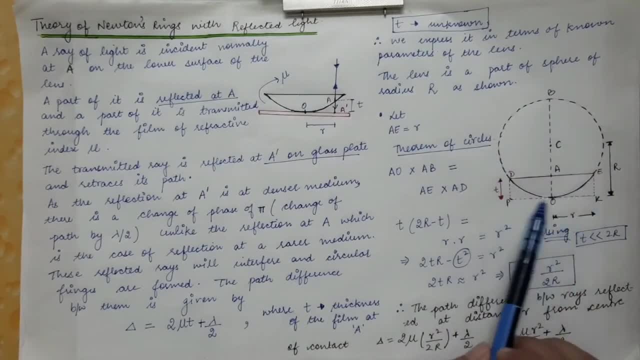 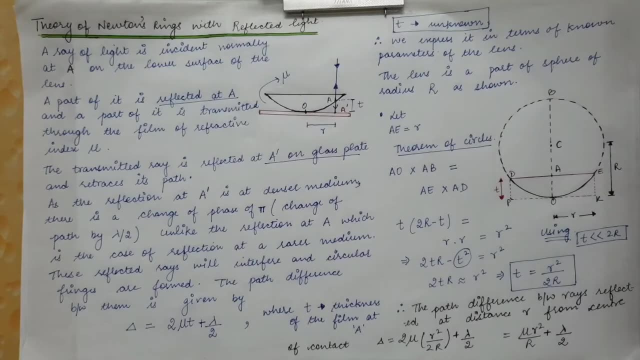 So what are the points which are at equal thickness of the air film of the sphere of which this lens is a part? Now a plane, no convex lens. it is a part of a sphere, of a particular sphere, because when we cut a small section from this sphere, we get a plane. 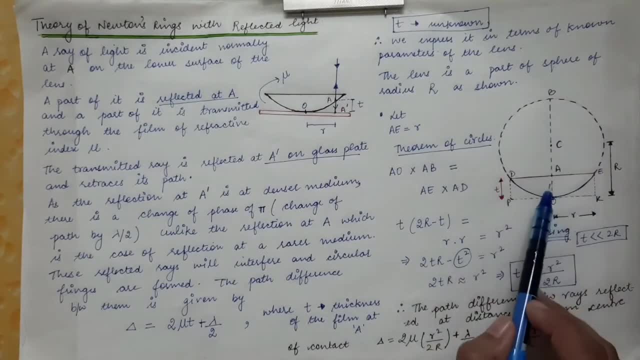 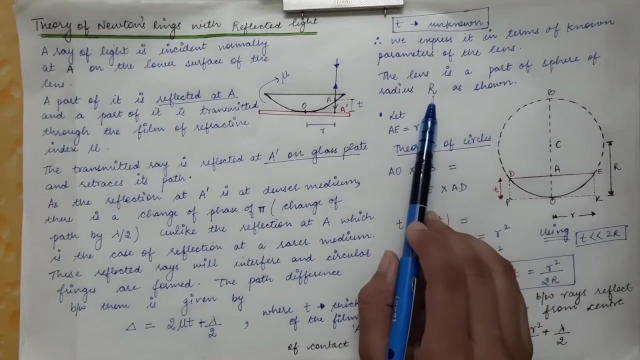 no convex lens. So this sphere of which this lens is a part, this sphere, it has a particular radius and that radius is called as radius of curvature and it is very easy to find this radius of curvature using a spherometer. So this radius of curvature, it can be found in the laboratories. 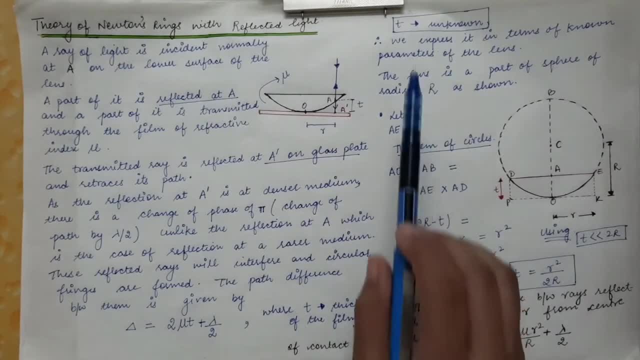 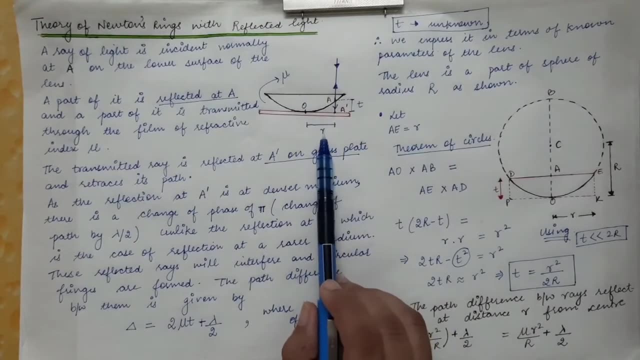 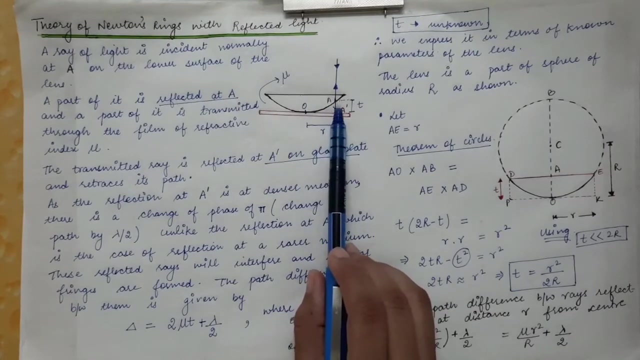 using a spherometer. Now we want to express this T in terms of capital R, and another parameter is small r. So small r it is the distance of this point from the point of contact. So at this point the thickness of the air film is small t and this point- same point- it is at a distance of small. 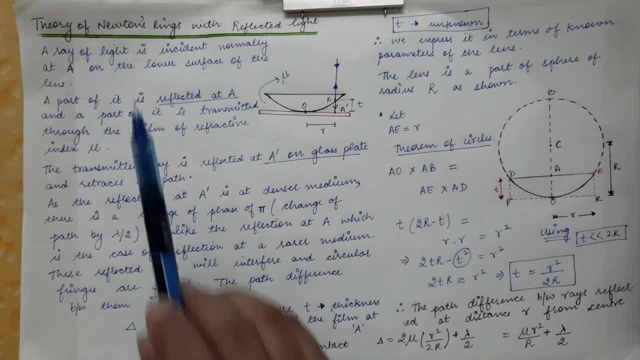 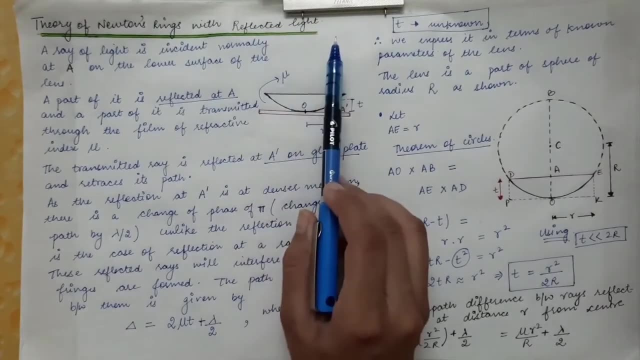 r. So this is the distance of the air film. So this is the distance of the air film. So this distance of the air film is small r from the point of contact, and we know that every fringe which is obtained over here, corresponding the, every fringe which is formed, it is formed. 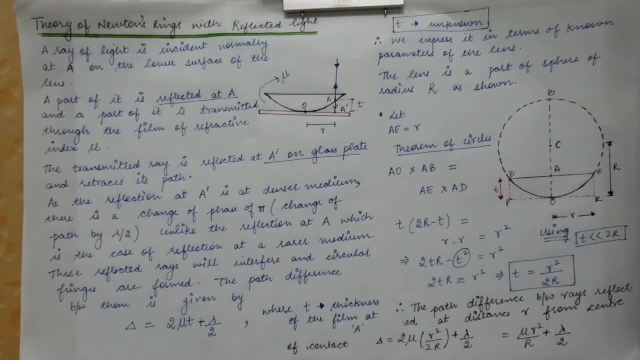 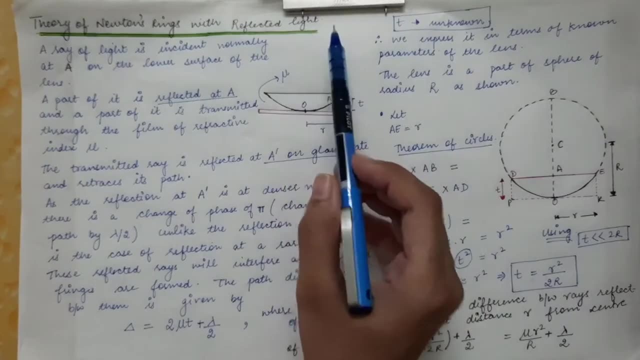 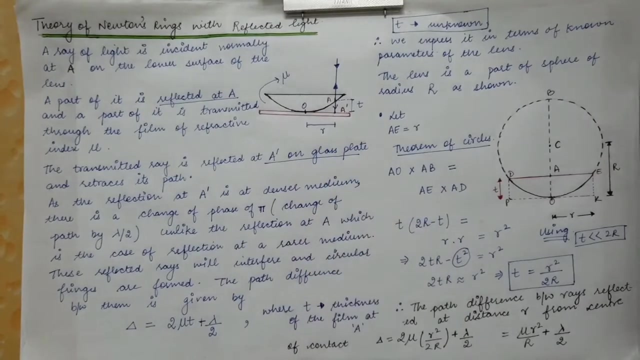 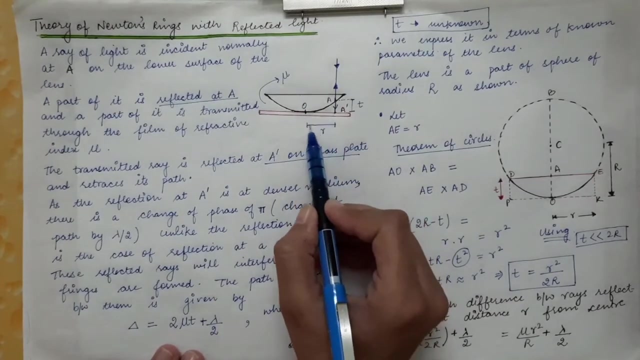 corresponding to the same thickness of the air film. So these are the thick, these are the fringes of equal thickness. So, corresponding to every fringe, there will be an equal thickness of the air film. So this are. it represents the radius of the circular fringes. So this is the distance of this point from the point of contact. and this distance, 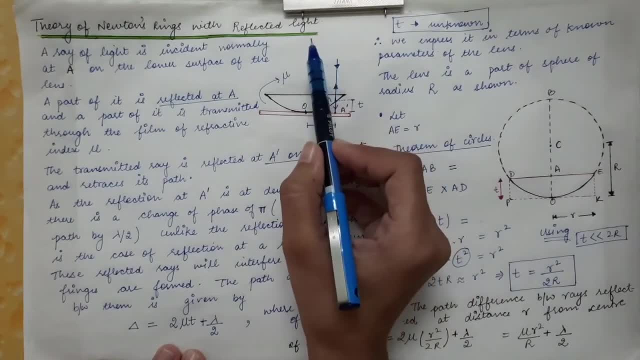 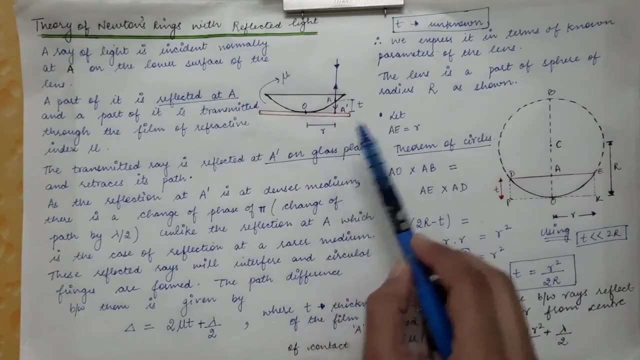 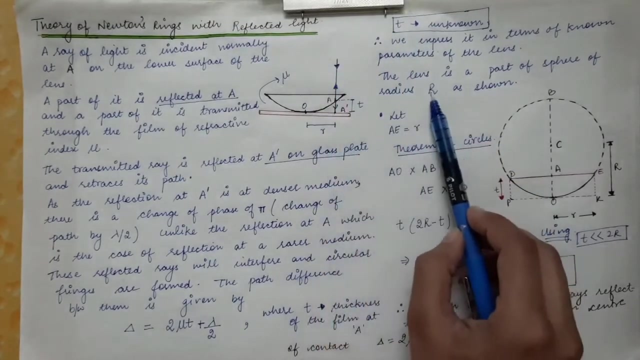 it will also correspond to the radius of the circular fringes. So now our main task is to find the expression of r, is to find the expression of T in terms of small r, which is the radius of the circular fringes, and capital R. So in this diagram we will use the 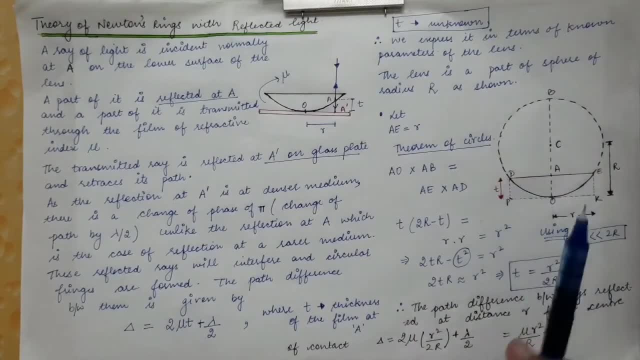 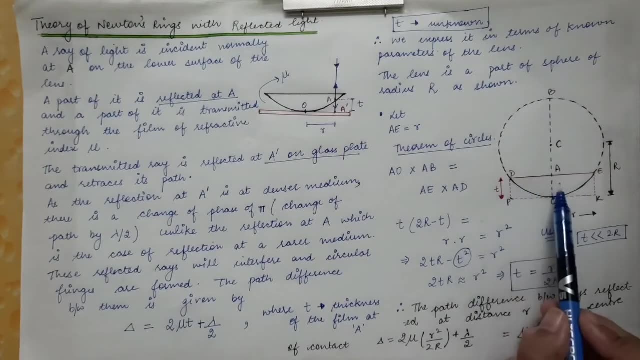 theorem of circles. So this is the length and the thickness we want to find. the expression of this is the thickness, small t and the distance of this point from the point of contact. let's say that is small r. So AE distance is small r and AD distance will also be equal to small. 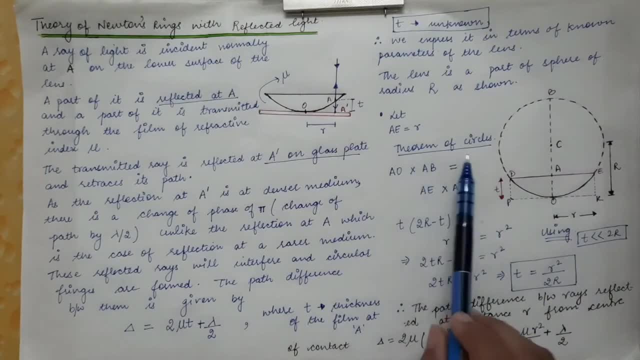 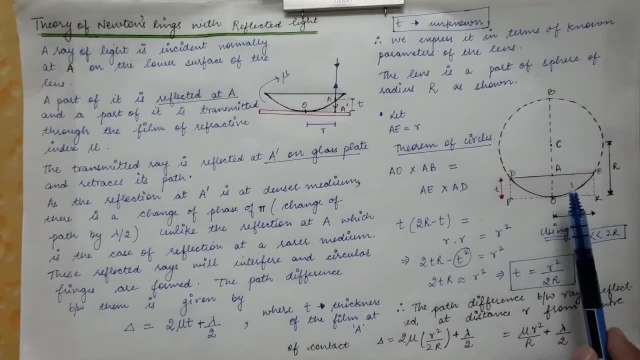 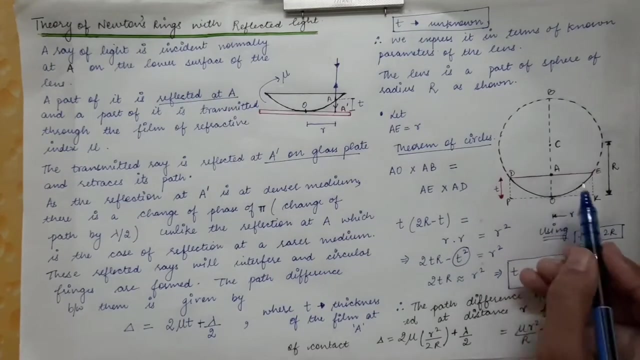 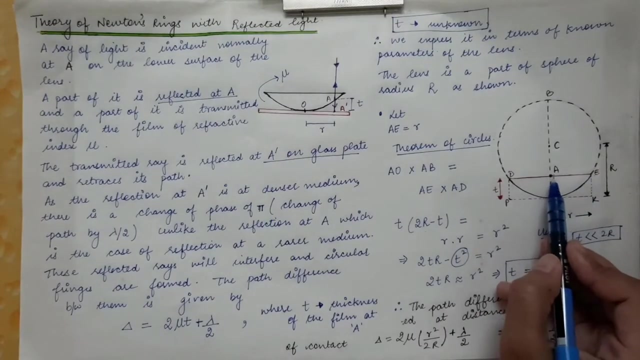 r. Now we will use the theorem of circle, which which tells us that AD in terms of small r is equal to small r. So AD into AE is equal to AO into AB. So at this point, so this theorem, it says AD into AE will be equal to OA into AB. So this is the theorem of chords, in case 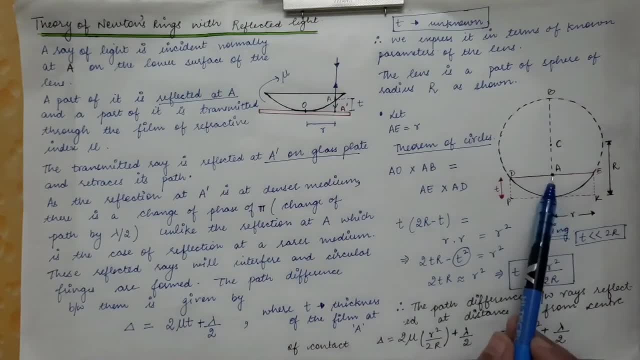 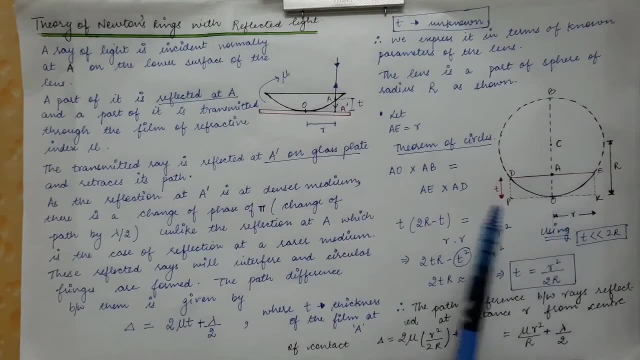 of circles. So now, what is AO? this AO, it is equal to thickness of the air film whose expression we want to find in terms of known parameter. So this is equal to T and AB, this whole AB. it will be equal to twice of r minus AO. So twice of r minus T, So AB will be equal to. 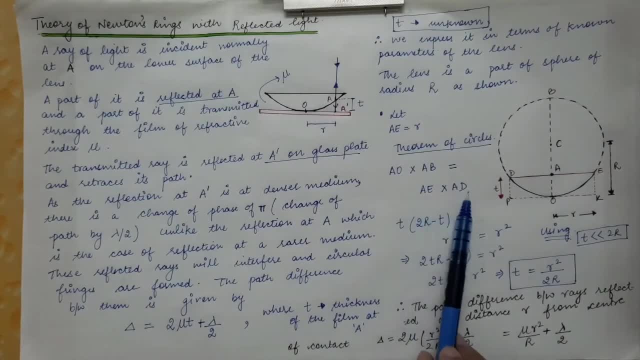 twice of r minus T and this will be equal to AE into AD, which is equal to small r. and we will also correspond to the radius of the circular fringes which are obtained in the travelling microscope. So in this case the thickness of the air film. it is very, very small as compared to 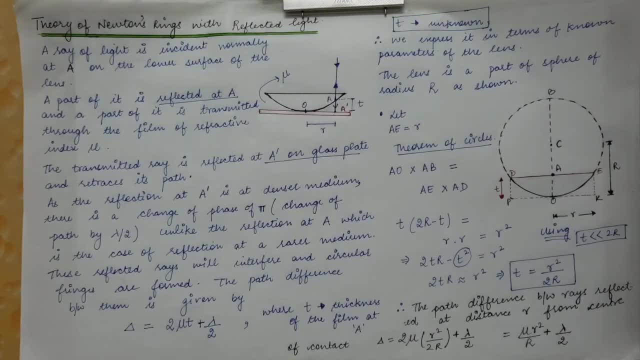 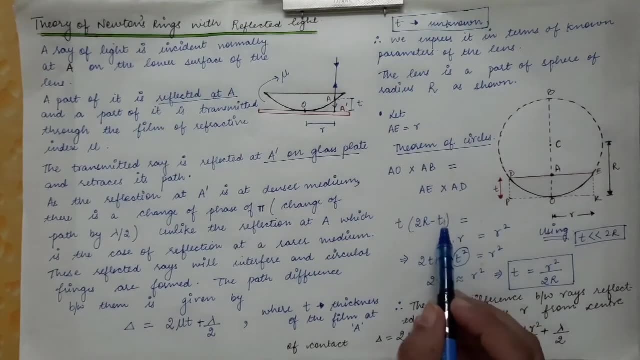 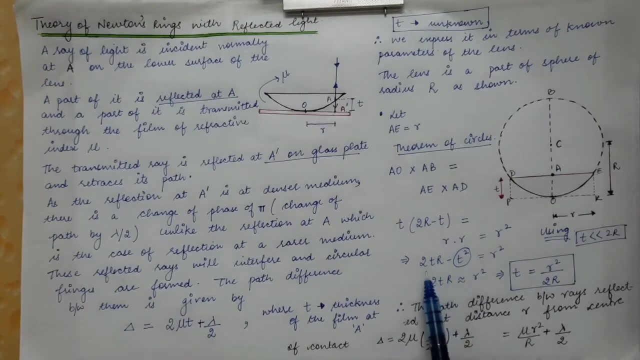 that of the radius of curvature. So T is very, very less as compared to twice of capital R. So over here T can be ignored. So T is negligible as compared to twice of capital R. So T can be neglected over here. So we will get: 2TR will be approximately equal to. 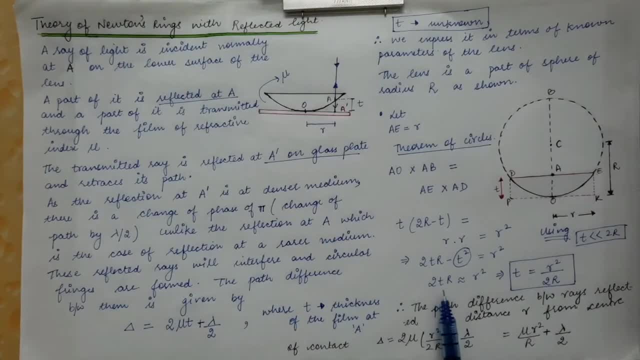 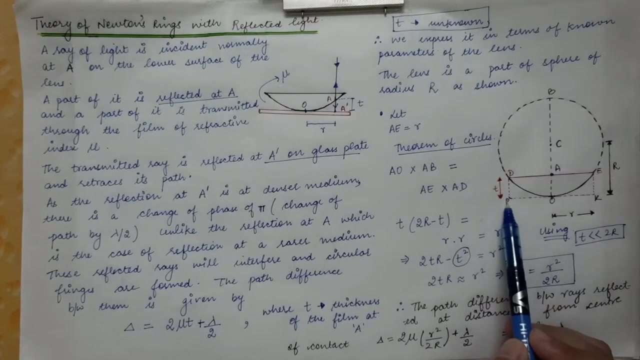 r square. So from here we can evaluate the expression of T. So T will be equal to r square divided by twice of capital R. So this is the expression of. this is the way of finding the expression of small t. the thickness of the air film in. 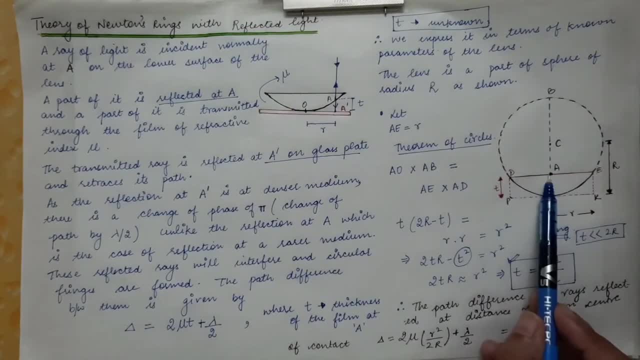 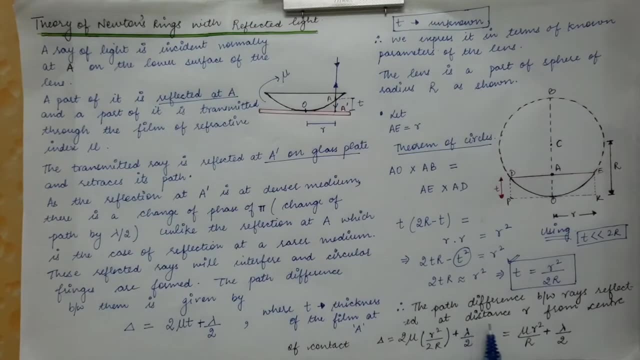 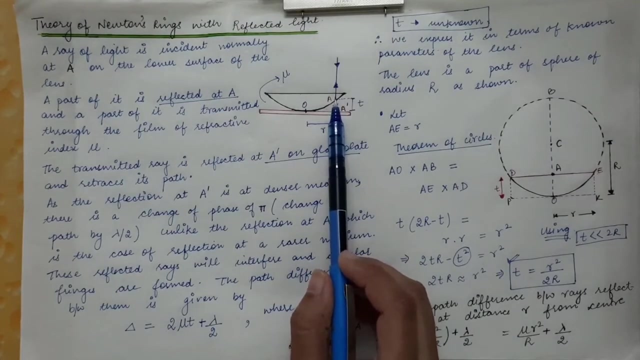 terms of its distance from the point of contact and the radius of curvature. Therefore, the path difference between the reflected rays at distance r from the centre, So the path difference between the radius of curvature and the radius of curvature. So this is the path difference between the reflected rays which are reflected at a point which is at 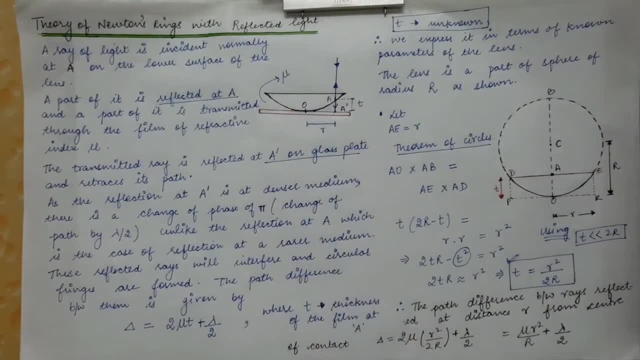 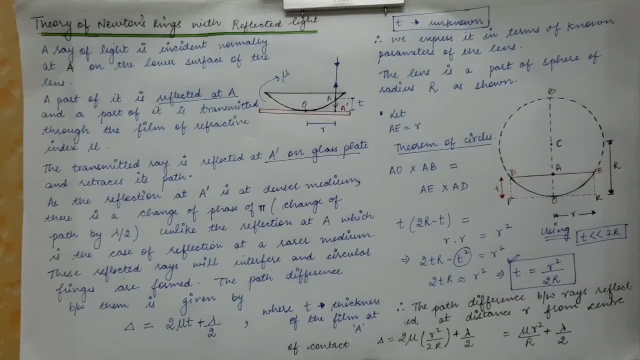 a distance of small r from the centre, So that path difference is equal to 2 mu t plus lambda by 2.. So now, in terms of T, we will put its value, which is 2 mu r square by twice of capital R plus lambda by 2.. So this will be equal to mu r square by capital R plus. 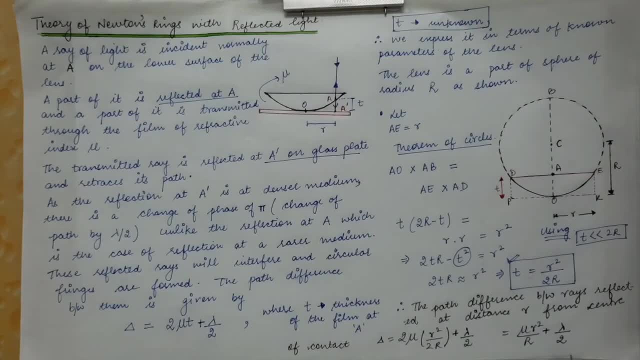 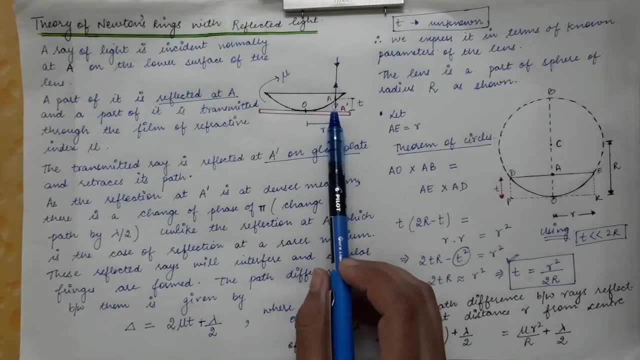 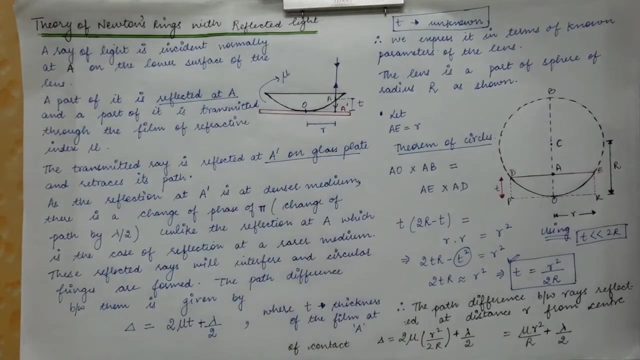 lambda by 2.. So this is the optical path difference between the two reflected rays which are reflected at a point of r distance from the point of contact, which are at a distance of r from the point of contact. So those reflected rays, they have an optical path difference which 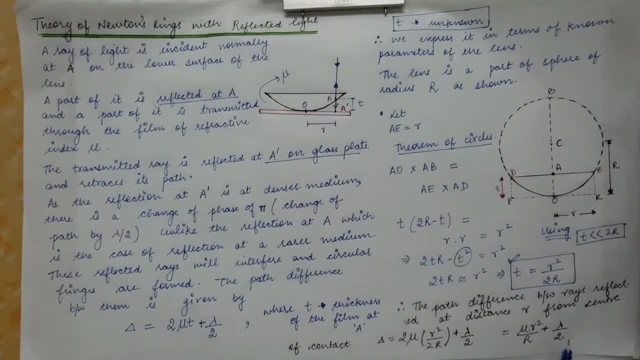 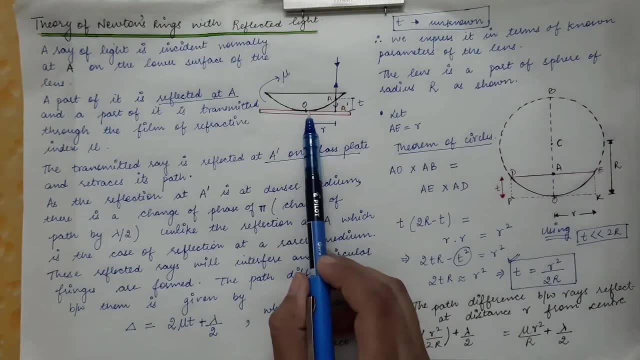 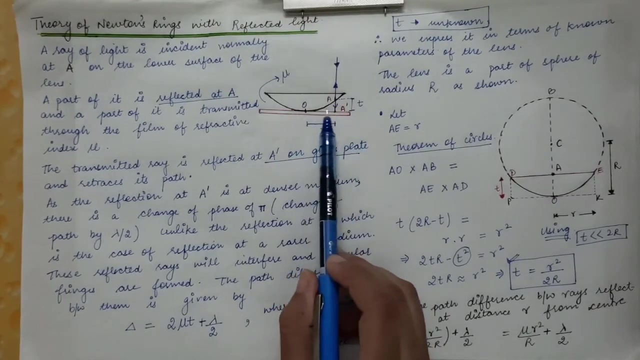 is given by this. So now optical path difference is given by this formula. So in this all terms are constant except small r. So as you will move away from the point of contact, the distance r, it will increase as you will go out of or as you will move away from the point of. 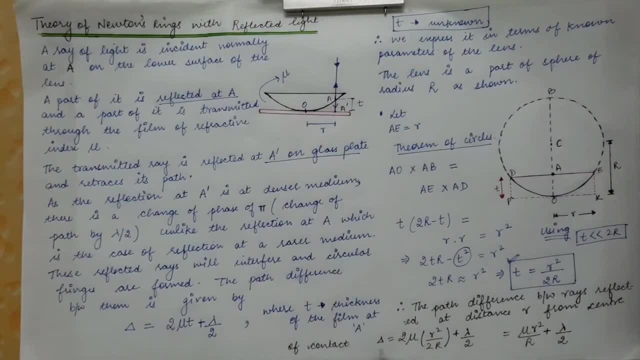 contact the r, it will increase. So the optical path difference will also change. Now, according to the value of optical path difference, if it is equal to n- lambda, we will get circular bright fringes, and when it is equal to n plus half lambda, we will get circular dark fringes. 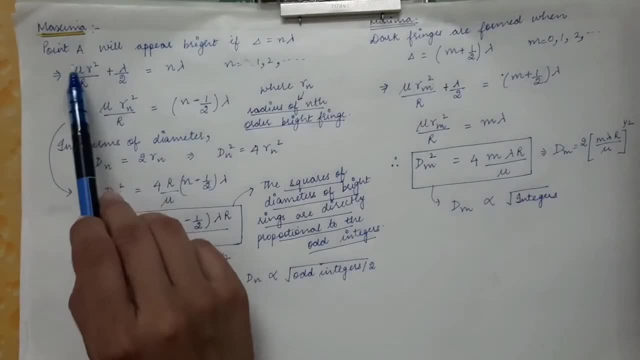 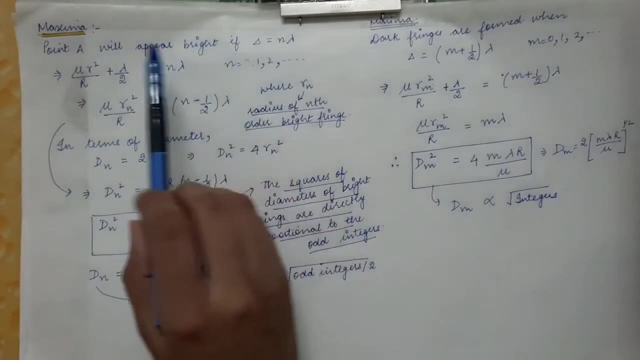 Now for the case of maxima, the point a that we had shown in the last diagram. the point a will appear bright if the path difference between the light rays which are reflected at point a and point a prime those reflected lights, if they will have a optical path difference of n lambda. So the circular fringes which 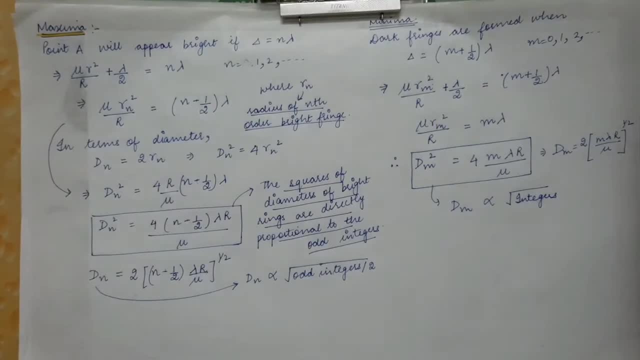 are obtained corresponding to this point, it will be a bright circular fringe. So optical path difference is equal to mu r square by capital, R plus lambda by 2, and if it is equal to n lambda, so then we get a maxima. So from here we can substitute by r n. So this represents: 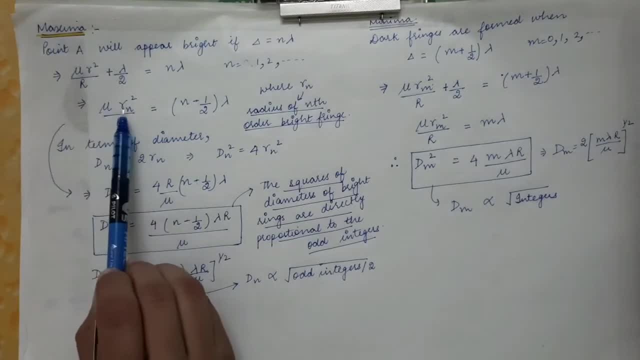 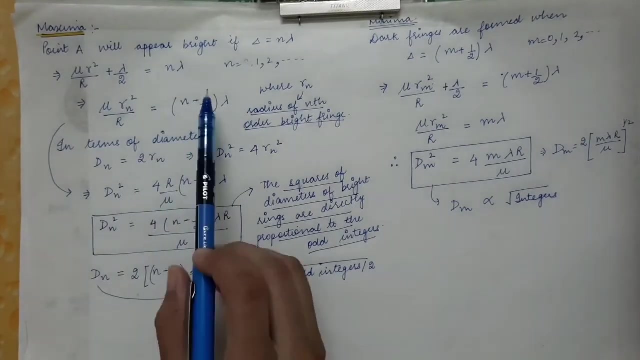 the radius of the nth bright fringe. So this r? n, it represents the radius of the nth bright fringe, and you can simplify this expression and you will get mu? r n square by capital, R is equal to n minus 1 by 2 times lambda. Now, over here, the n will take the radius of. 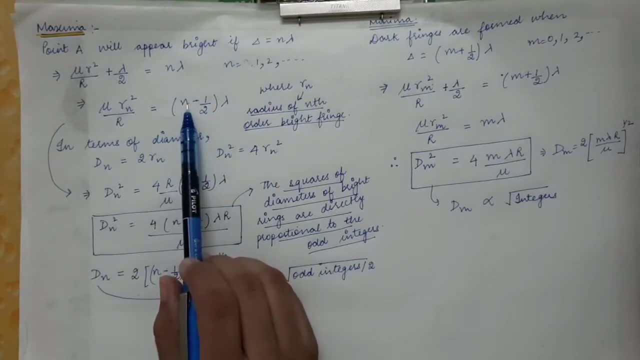 1 by 2 times lambda. Now here the n will take the radius of 1 by 2 times lambda. Now the values from 1,, 2,, 3,, 4.. Now n will not take a value of 0 because if you will put n is 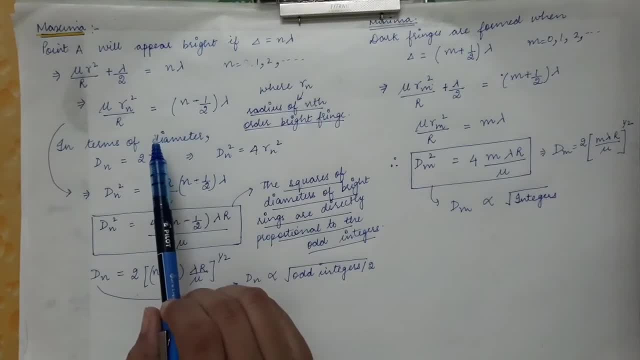 equal to 0. so on the right hand side you will get minus lambda by 2, whereas on the left hand side all the parameters, they are positive, So n- it cannot take value is equal to 0 in this particular expression. Now we will substitute the expression of Rn in terms of its diameter. 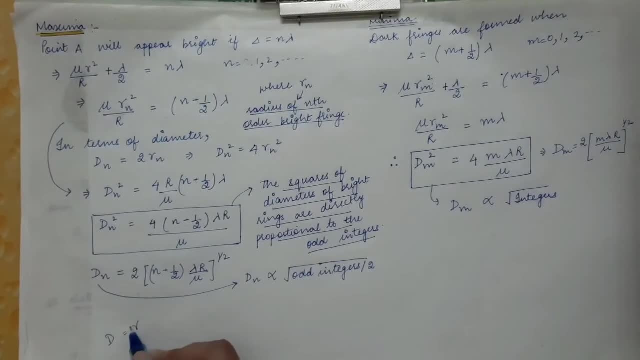 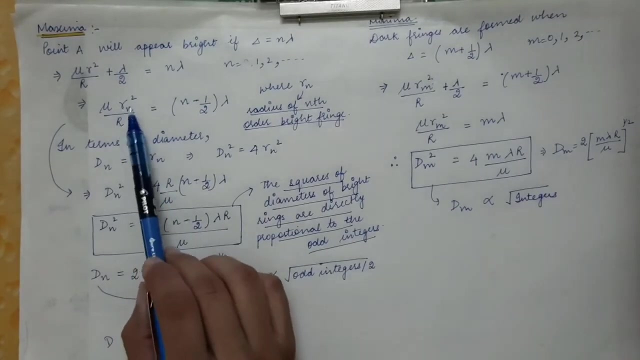 Now the diameter is equal to twice of R, twice of the radius, So d square will be equal to 4 times R square. So from here you can find R square will be equal to d square divided by 4.. So we can substitute Rn square in terms of dn square, So dn will represent the diameter. 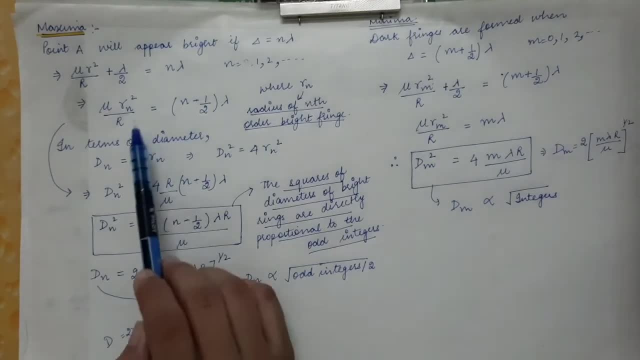 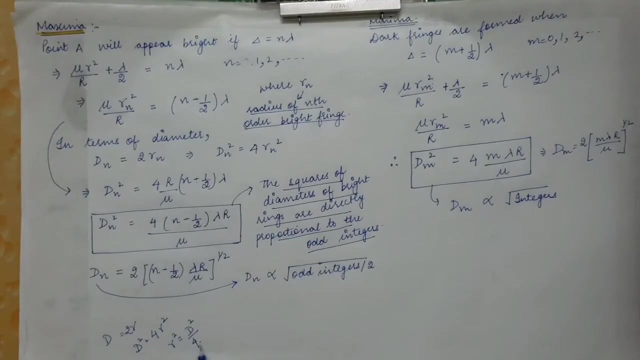 of the nth bright fringe, So we will get dn square. So dn square it will be equal to 4 times capital Rn minus half times lambda divided by mu. So from this expression, if you will put Rn square as dn square by 4, so you will get this expression. 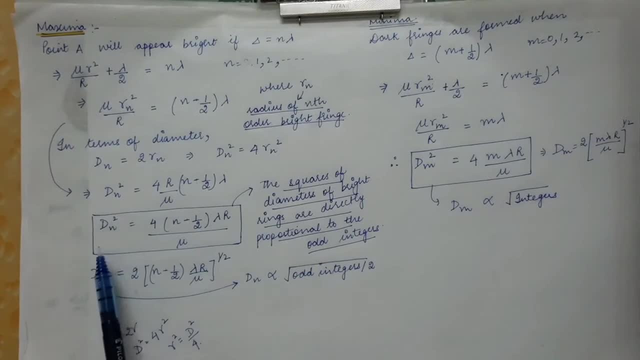 of the square of the diameter of the nth circular bright fringe, So the squares of the diameters of the bright rings. they are directly proportional to the odd integers and the diameter it can be evaluated by doing the square root on the both sides. So you will get this expression. 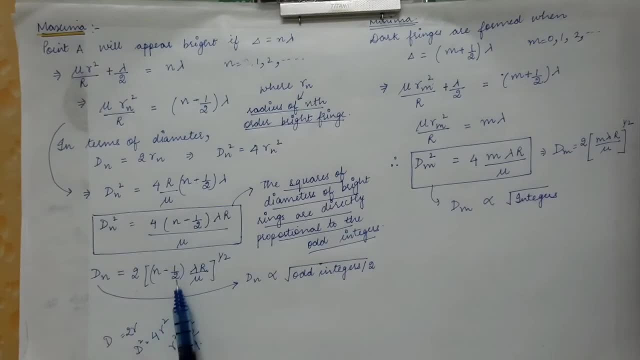 and inside this square root we have n minus half. So the value of n is equal to 1. lower value of n is equal to 1.. So you will get 1 by 2, then you will get 3 by then you will get 3 by 2, then you will get 5 by 2, and so on. So the diameter of the nth bright circular. 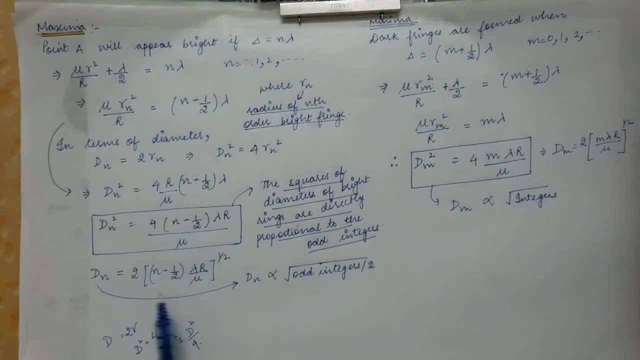 fringe. it is proportional to odd integer divided by 2. Because we are getting over a square here. 1 by 2, then you will get 3 by 2, then 5 by 2, then 7 by 2.. So this is proportional. 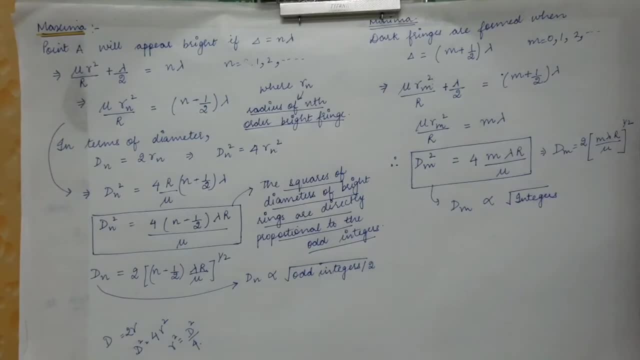 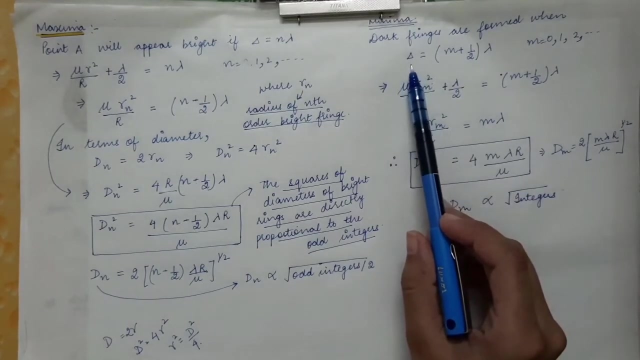 to the square root of odd integers divided by 2.. Similarly for the case of minima, So the dark fringes. they are formed when the optical power difference is equal to n plus half lambda. Now this m, it will take values from 0, 1 to 3.. So delta, it is the optical 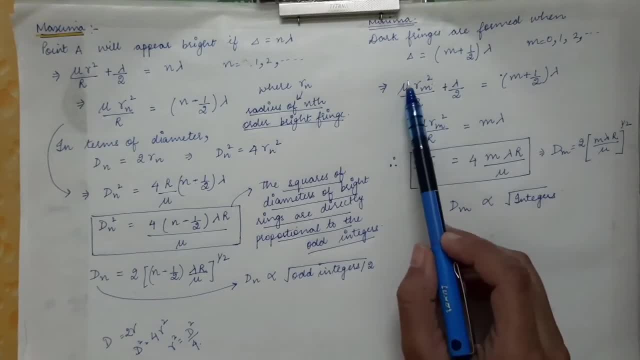 power difference. So optical power difference: we have already evaluated it is equal to mu times Rn square by capital Rn. So this is the optical power difference. we have already evaluated it is equal to mu times R plus lambda by 2.. So this is the optical power difference. 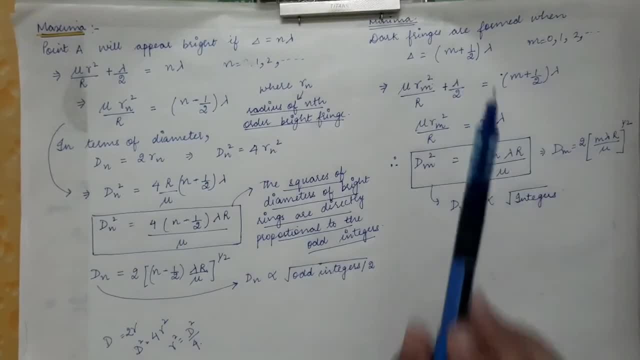 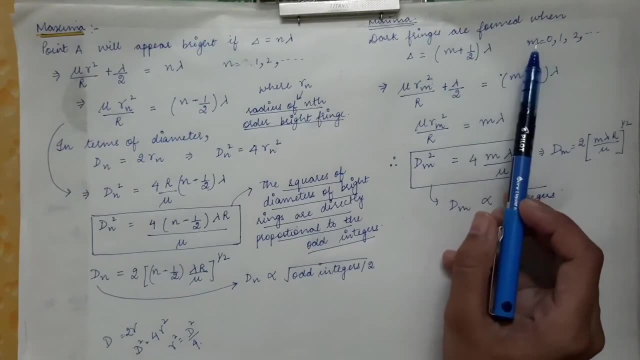 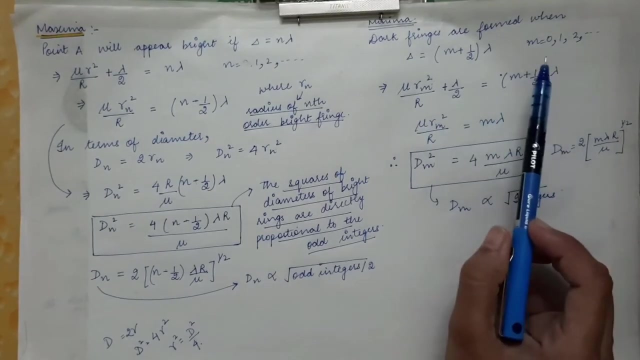 and when this is equal to m plus half lambda, then dark fringes are obtained. Now, over here, the minimum value of m 0, that is, m is equal to 0, is possible in this case Because when you will put m is equal to 0, you will get a positive term on the right hand side and 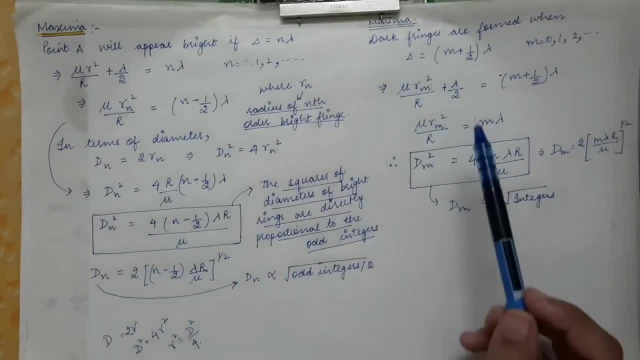 we also have positive terms on the left hand side. So, on simplifying this expression, you will get mu Rn square by 2.. So this is the optical power difference, and when this is equal to m plus half lambda, then dark fringes are obtained. Now over here, the minimum value. 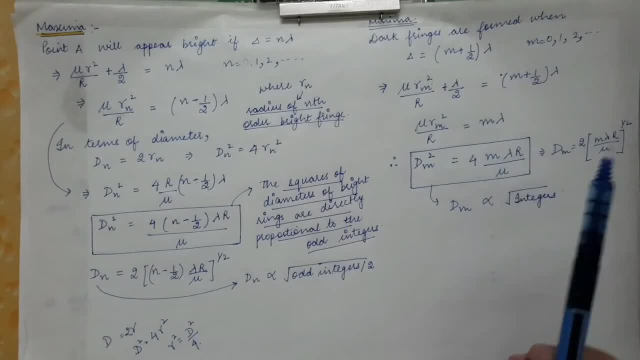 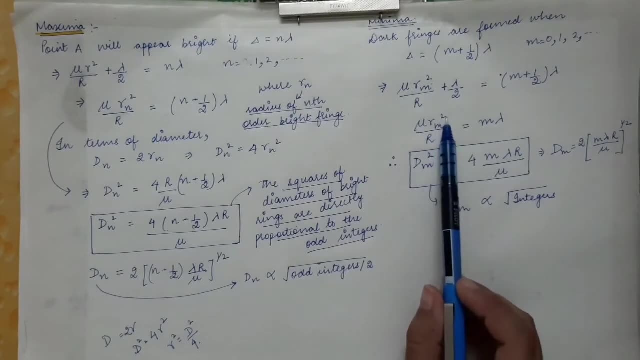 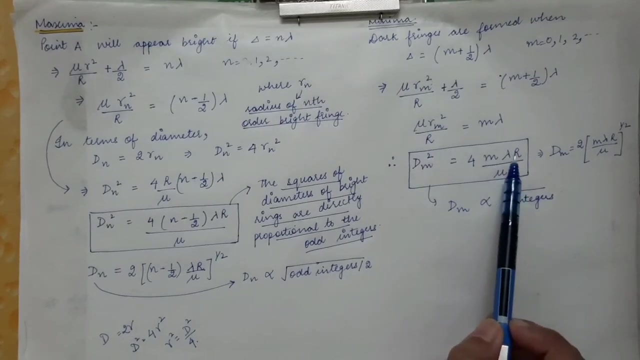 of m square by capital R is equal to m lambda, So from here you can find the diameter of the mth dark fringe. that will be equal to. you will substitute Rn square by dm square divided by 4.. So you will get dm square is equal to 4 times m lambda capital R divided. 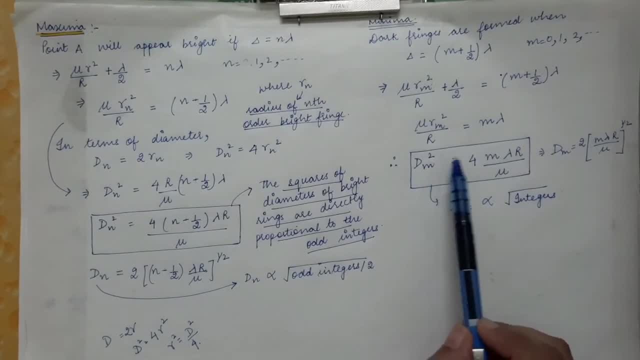 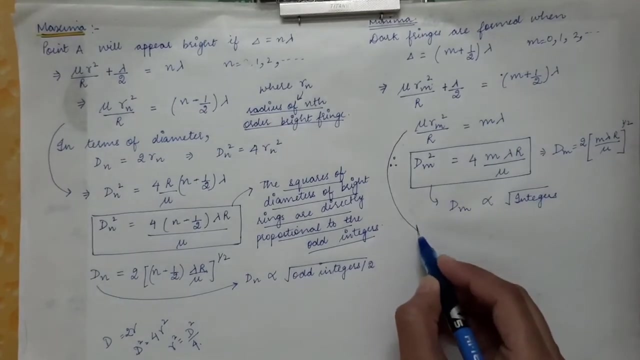 by mu. So from here you can find the expression of dm by doing the square root on the both sides. Okay, now in the enumZe Senhor. so here I am taking, adding in the important values: m. We want to exceed this equal to 8, because we are going to be Поэтому worth. 5 meters high. So I am taking integral values which will increase or decrease by 2.. So this is we want to exceed, and then it is going to be paintings. so f is equal to f, but in this case it will be a matrix localized antir�um which goes to the a�ry of the omn. it will be is equal to 0.. Now, on the clearing spectrangular value of of Pr milk mango which, with an altitude of MÖ 0.. So dm then we have the potential. m is equal to m plus half lambda. So anesthetic for the dark fringe, it is proportional to the square root of integer. here it is the. 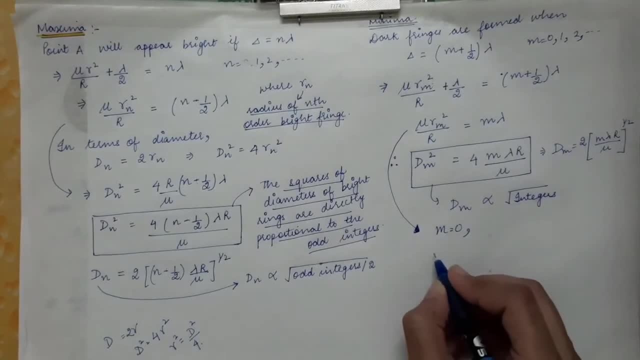 m, it take integral values, so hisア, it is proportional to the square root of integers. now for the case of minimum. Now, So for m is equal to 0, we will get mu rm square divided by capital, R will be equal to 0.. 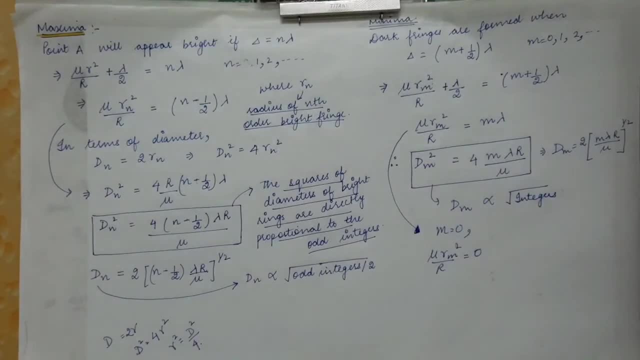 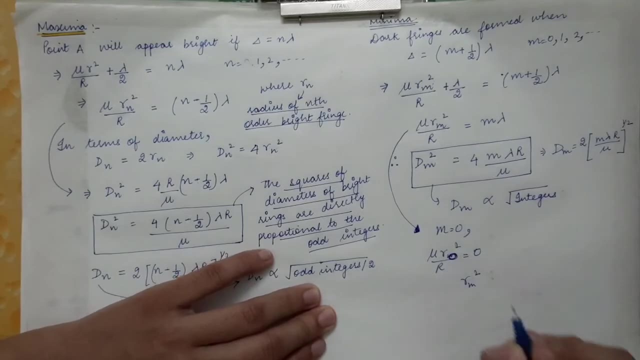 So when you will put m is equal to 0, so mu rm square divided by capital R, it will be equal to 0. So means the rm square, or you can say r0, we are putting the value of m is equal to 0.. 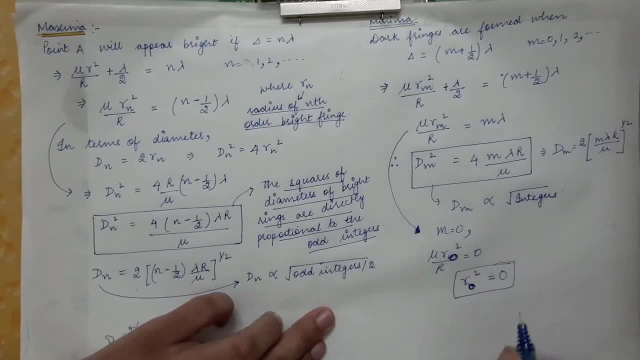 So r0, it will be equal to 0.. So this is the radius of 0th order, dark fringe, And from here we have seen that when you will put m is equal to 0, the radius will come out to be equal to 0. 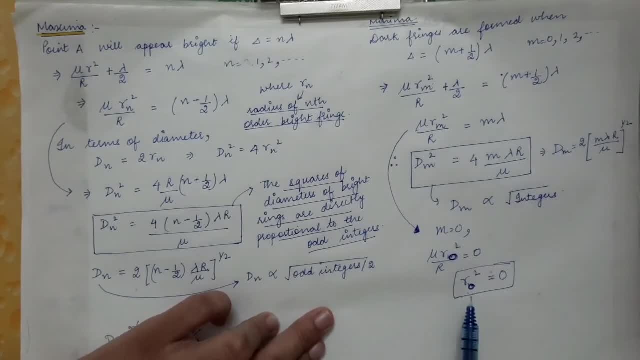 And radius is 0 for the central fringe. So for the central fringe now, what is r? r is the distance of the point from the point of the contact. So r is the distance of this particular point, of any point on the thin film, from the point of contact. 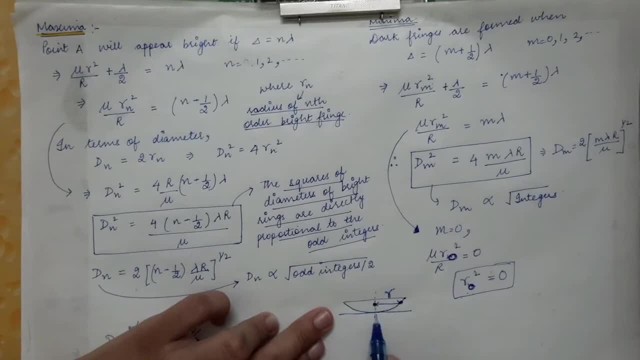 So, when r, r is equal to 0.. r is 0 at this point, At this point of contact, At this point of contact which is shown by a cross. So, at this point of contact, r is equal to 0.. 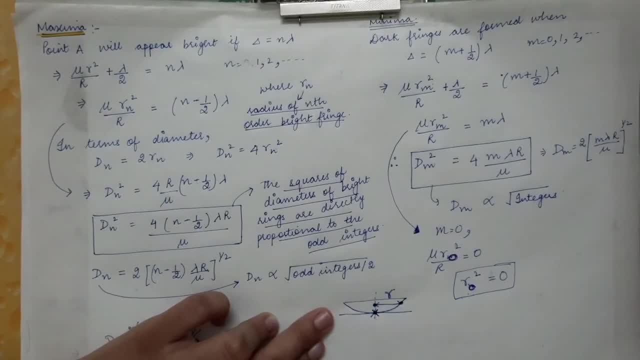 And the lights which get reflected from this point, they make a central fringe. So lights which fall on this point and get reflected, they will form the central fringe. So what is the nature of the central fringe, If it is a dark fringe or it is a bright fringe? 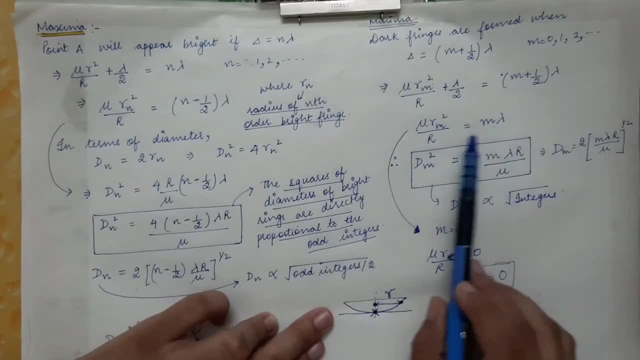 So, in the case of When you will put, m is equal to 0. So you get r. 0 is equal to 0. So the radius of the 0th order, dark fringe, it comes out to be equal to 0.. 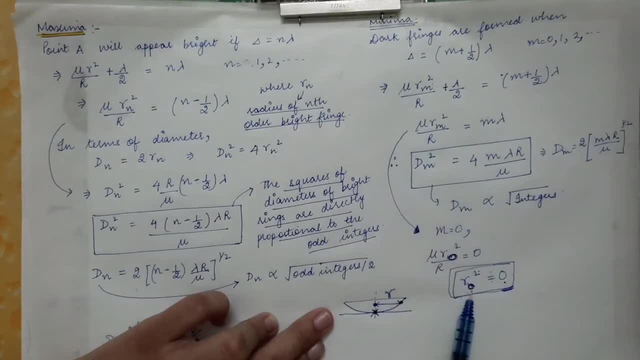 So from the condition of minima we get the radius of the 0th order dark fringe. it comes out to be equal to 0. So means at r is equal to 0. At r is equal to 0, we get a dark fringe. 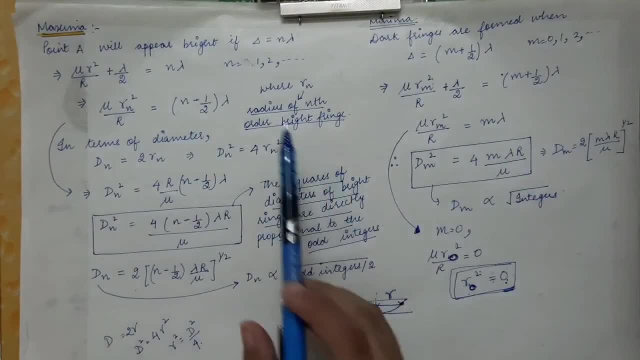 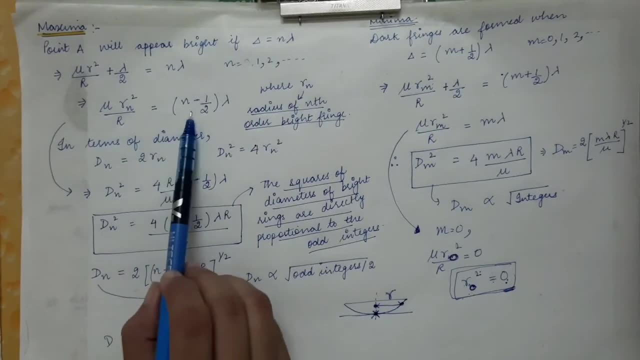 Whereas in this case, In the case of When you will put n is equal to 1.. The minimum value of n is equal to 1.. So when you will put n is equal to 1 in this expression, So when you will put n is equal to 1.. 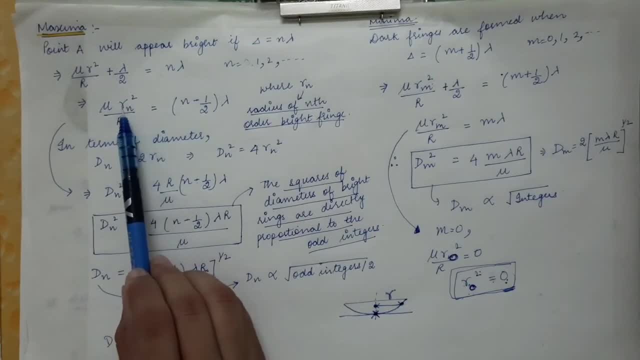 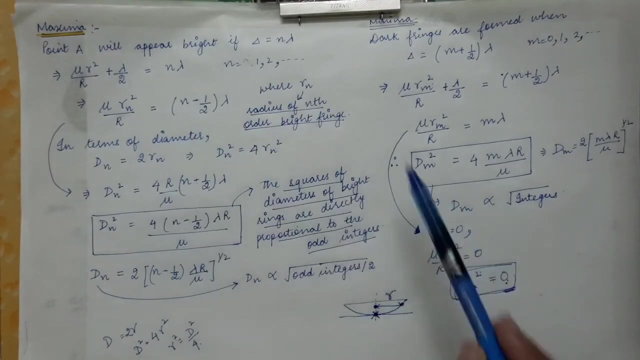 You will get a finite number or finite value of the first bright fringe. So you will get a finite value of the first bright fringe. So the first bright fringe it is formed at some distance from the point of contact, Whereas the first dark fringe 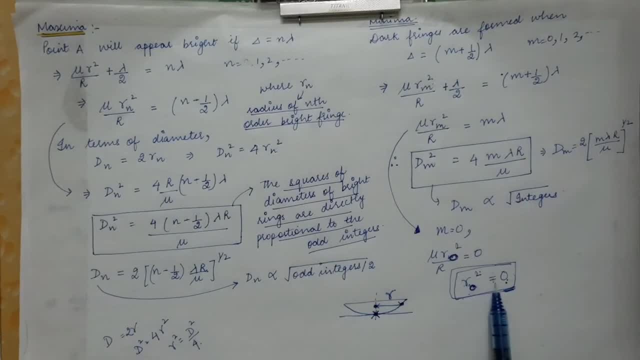 Or the 0th order, dark fringe. it is formed at r, is equal to 0. Means at point of contact. So the central fringe for the case of thin film, If the thin film is air, So the central fringe for the air thin film. 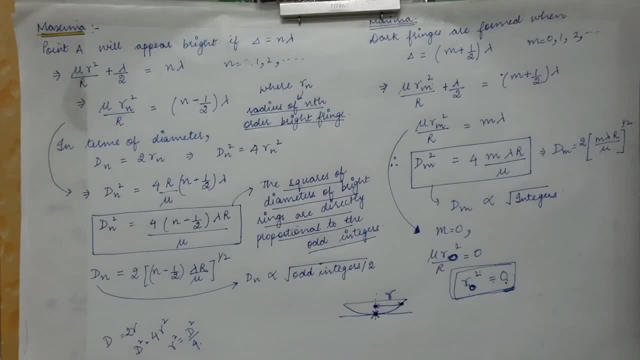 In case of Newton's rings, it is a dark fringe. 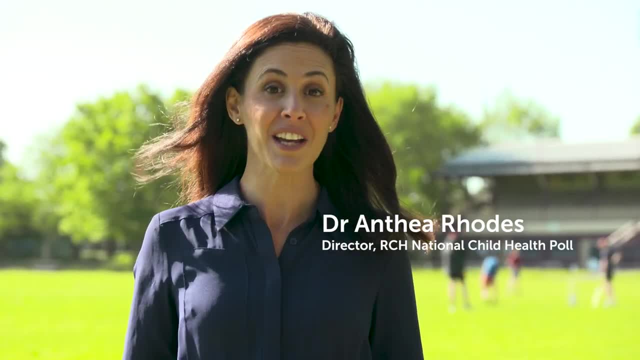 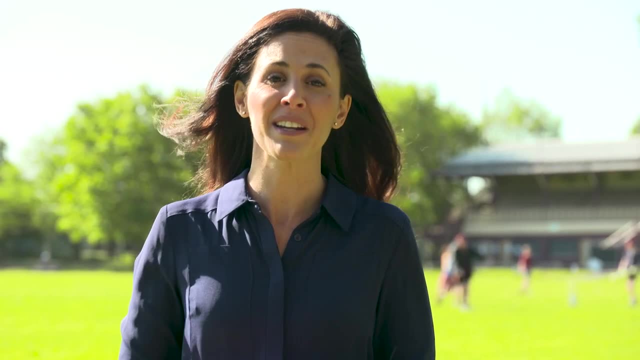 Hi, I'm Dr Anthea Rhodes, paediatrician and director of the RCH National Child Health Poll. In our latest study, we found that more than half of Australian kids have participated in less organised sport and physical activity since the start of the pandemic. 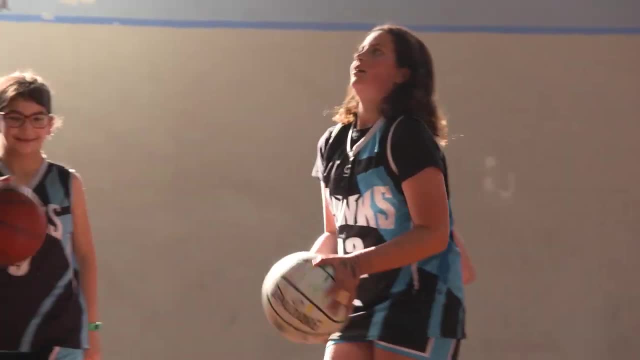 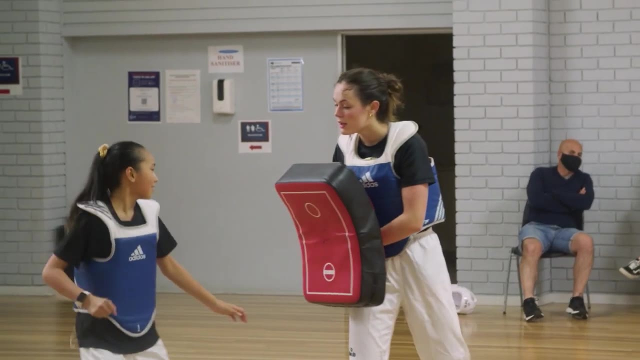 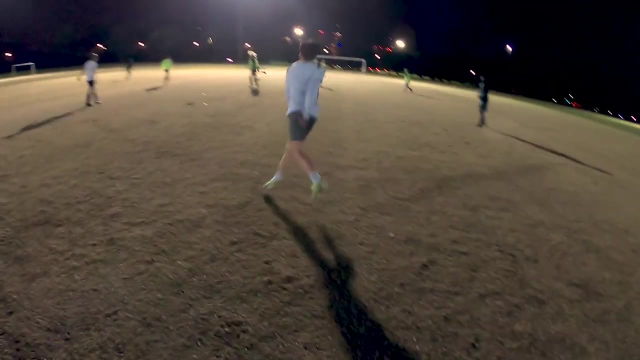 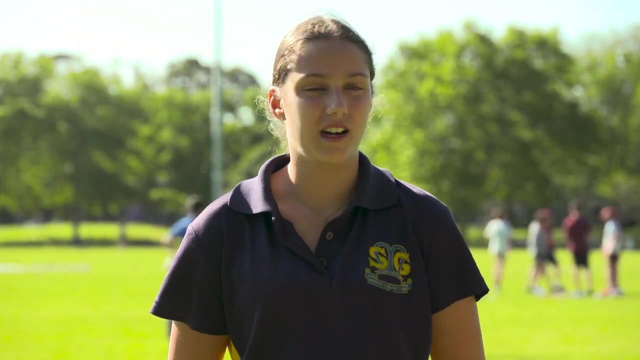 As restrictions ease across Australia, it's important to encourage children and families to return to community sport and organised physical activity. I just missed the drives at 7 o'clock in the morning to footy games. I missed the lollies snakes at half time.